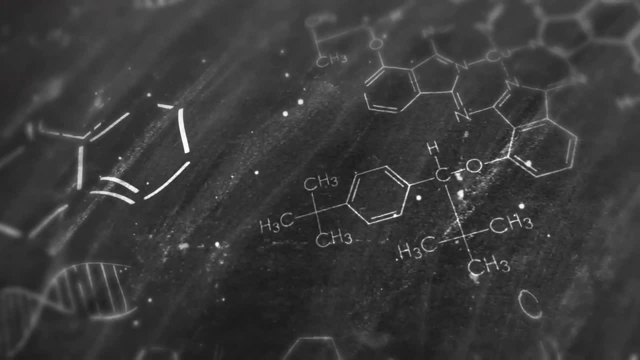 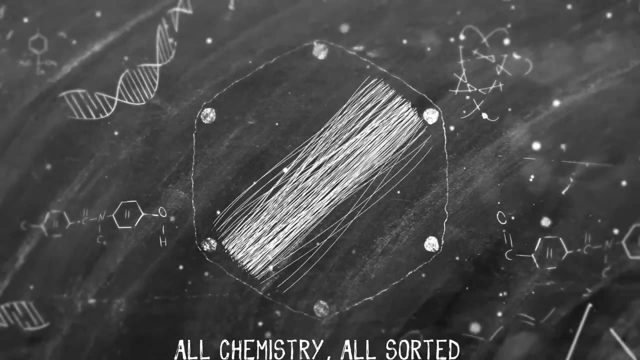 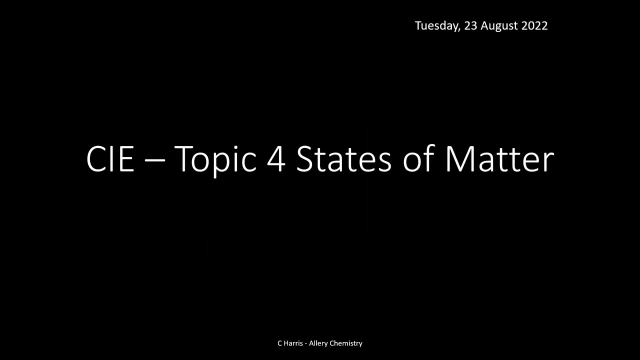 Hello, my name is Chris Harris and I'm from Allery Chemistry, and welcome to this video on topic 4, States of Matter. This is for the CIE topic, so this is the Cambridge Internationals paper. So obviously in this topic, as it suggests, we're going to look at states of matter. so 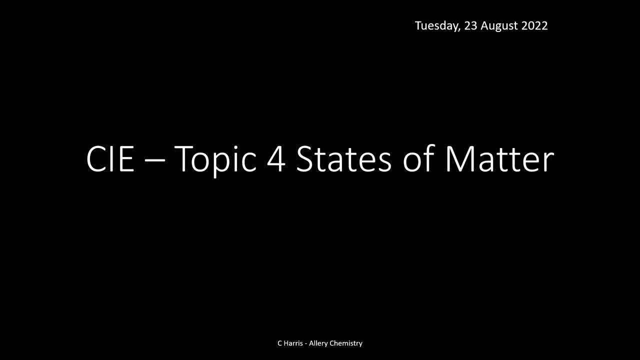 solids, liquids and gases and just kind of A-level it a little bit and kind of put some extra bits of information in there. So obviously that's the focus of this. It is obviously dedicated to the Internationals qualification, so if you're studying that, then this is the. 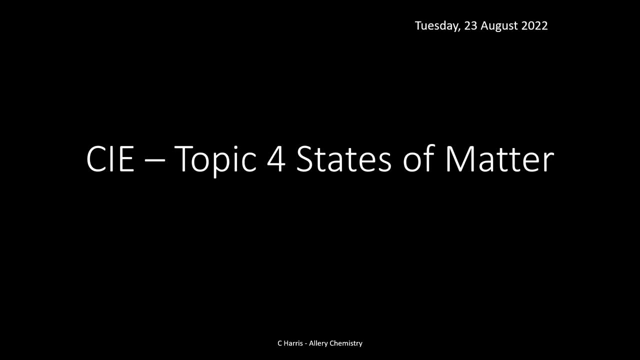 right place you need to be. These slides here are available to purchase if you wish to purchase them. They're great for your revision on the go or, you know, for you to look back in your own time. If you just click on the link in the description box below, you'll be able to get. 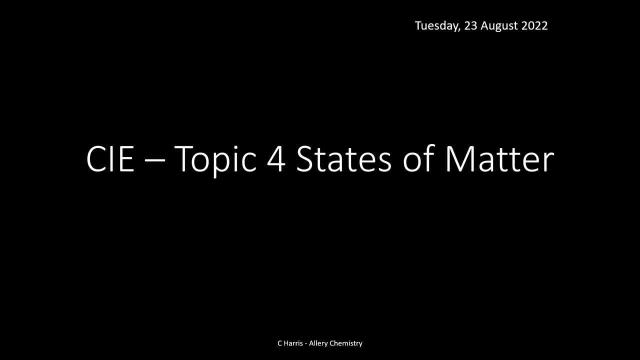 a hold of them there. They're great value for money and I've bundled them together as well into the different topics. So, for example, this falls into the physical chemistry topic for year one, so I kind of bundled it there. but you can get the full range if you want for year one and 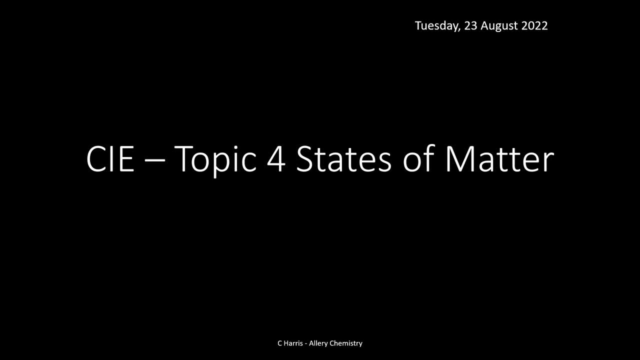 year two. Okay, so without further ado, let's crack on. So I'm going to look at states of matter first and let's have a look at an introduction. Now you might be looking at this really easy this: you know: solids, liquids and gases. It's about what you did, you know. 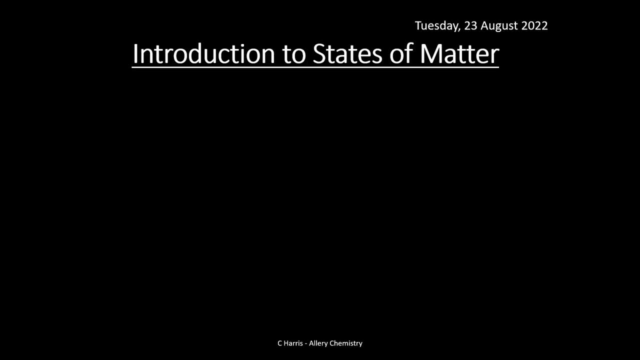 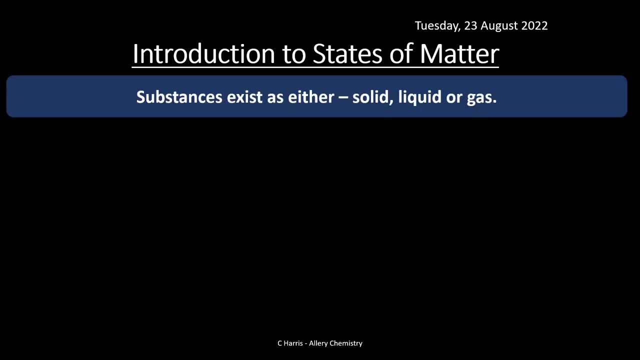 when you were 11, probably even earlier than that, I would imagine. But this is going to be a little bit trickier and you'll see there's extra little bits that you need to be aware of And obviously, at A-level, you've got to make sure that you're using your key terms. I know you have to do it. 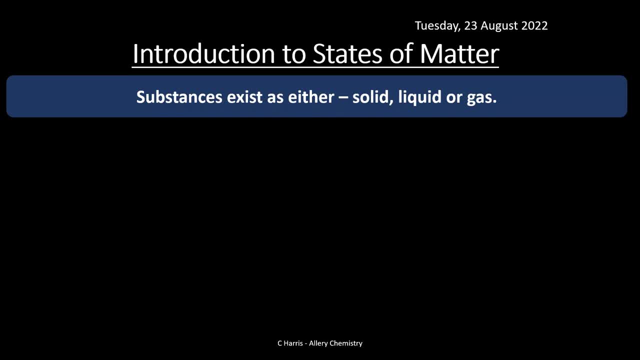 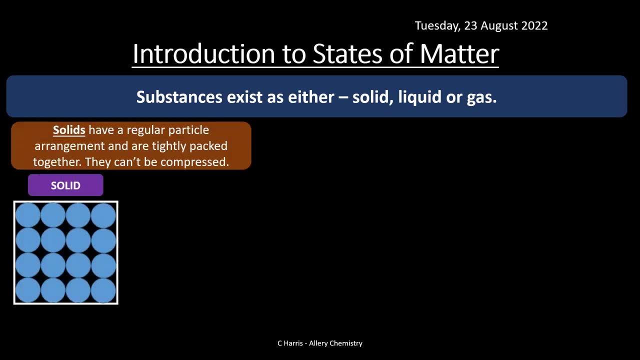 in GCSE as well, but at A-level in particular, you've really got to be precise and talk like a scientist, I suppose. So let's have a look. So obviously they exist as solids, liquids and gases, so we know that. 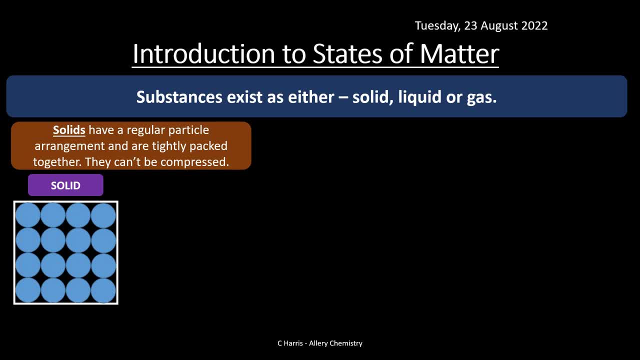 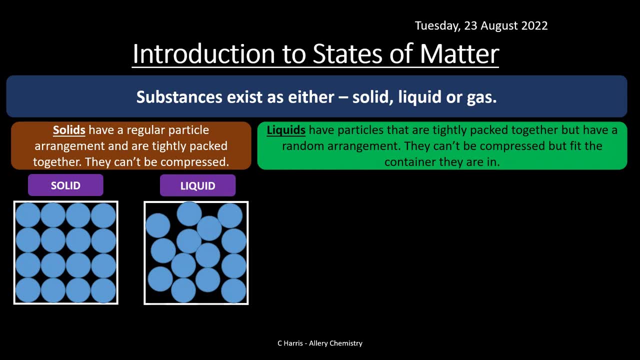 And solids have a regular particle arrangement. they're tightly packed together and they can't be compressed, as you're probably aware of that. Liquids: they are not tightly packed together. they do have a bit of a random arrangement. So they are tightly packed together. they have a 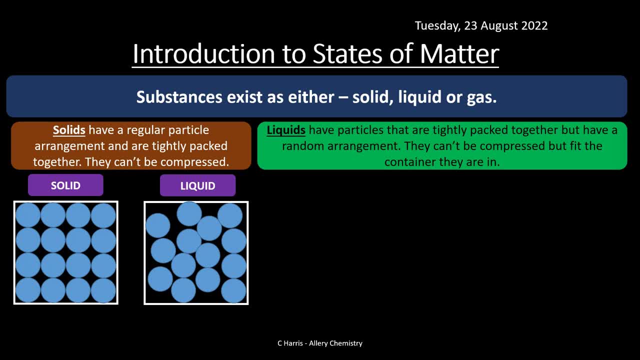 random arrangement. That's not a good start, is it? So they are tightly packed together, definitely. If you try and put that in a syringe, you won't be able to squash that, And they obviously fit the container they're in And gases have a random arrangement. 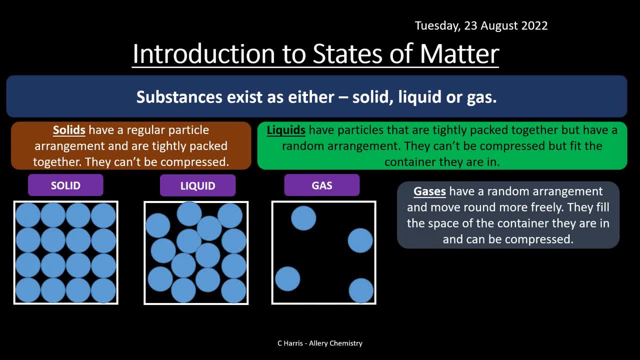 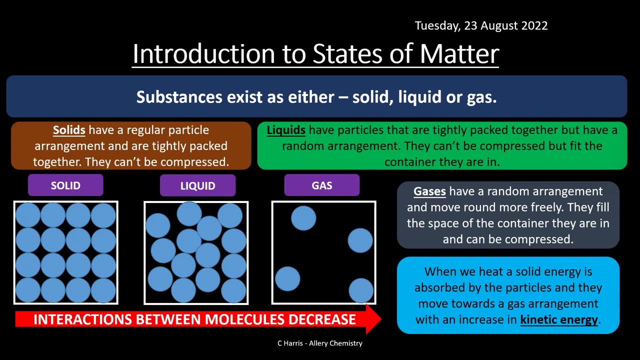 so they do have a random arrangement. They fill the space that they occupy, they move around freely and they can be compressed. So if you put that into a syringe and put your thumb over the end of it, then you'll be able to squash the gas. And so obviously, when we heat a solid, for example, 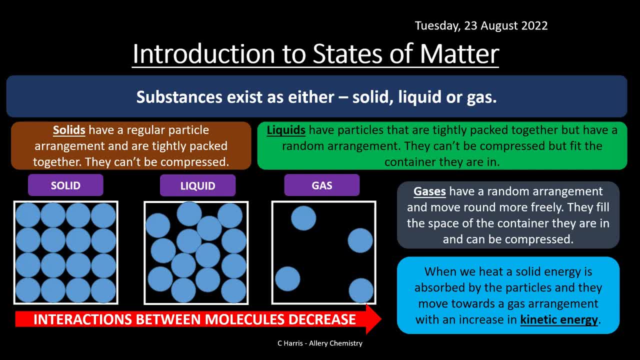 then heat is absorbed by the particles and they start to move more and more and more and they vibrate much more vigorously- And we'll see a heat profile graph later on in this video- And they move towards a gas arrangement Because they have more kinetic energy. So that's basically how we get from solid liquid to gas. 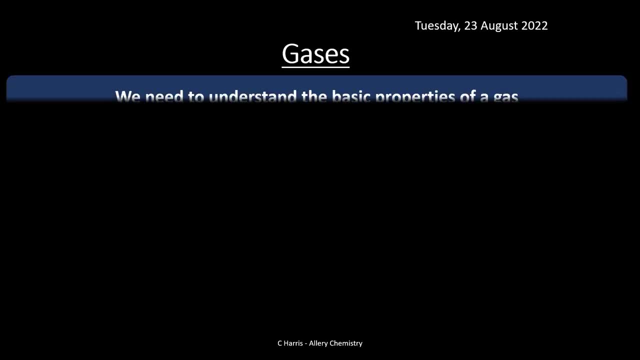 Okay, so let's start looking at gases here. Now this is where it gets a bit technical, So I did warn you it might be a bit difficult. It's not too difficult, it's alright, But it's a bit more advanced than what you're normally used to. 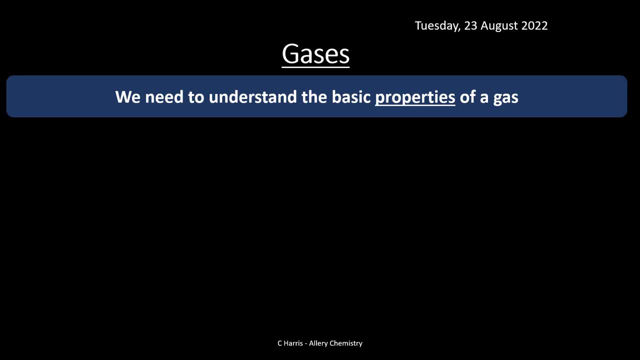 So we need to understand the basic properties of a gas first, And you'll never look at a gas in the same way again after you've gone through this. So we have a low density, okay, and that's due to the fact that the particles are obviously spread out. 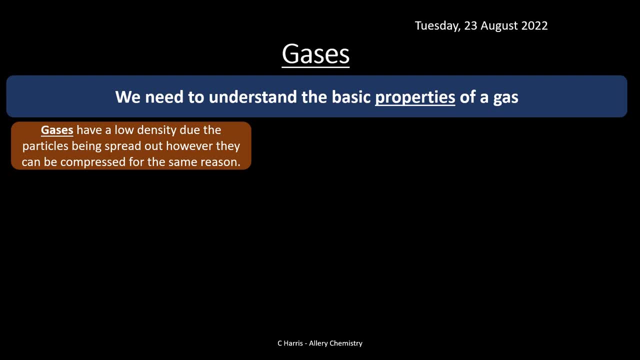 However, they can be compressed for the same reason. Because they have a lot of space between the particles, then we can compress them. They don't have strong attractions to each other and so they fill the container. they're in quite well. So this kind of feeds in from the previous topic, topic three, when we looked at intermolecular forces. 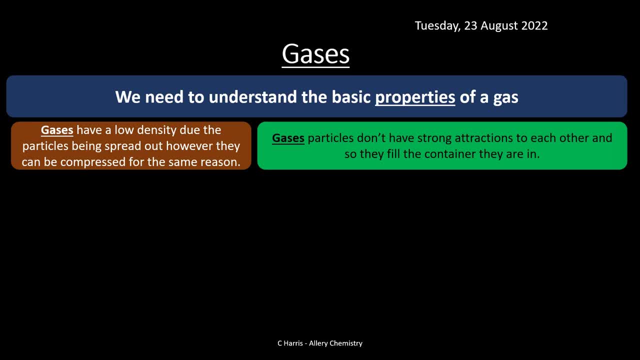 So you'll find a lot of the CIE topics. they kind of merge one to the other So you'll see there'll be bits in here where I've kind of pulled it from topic three. So yeah, so don't be kind of alarmed if you watch topic three and think I thought he's just said that. 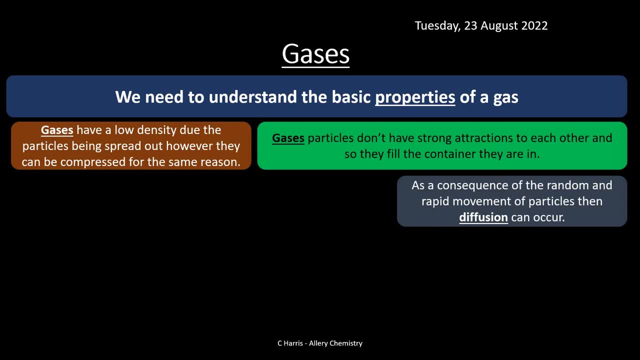 Is that got deja vu? And actually, yes, it is basically. So there's a lot of overlap between them. So, yes, you'll probably see some similarities here. But as a consequence of the random and rapid movement of the particles, then we can have a phenomenon called diffusion. 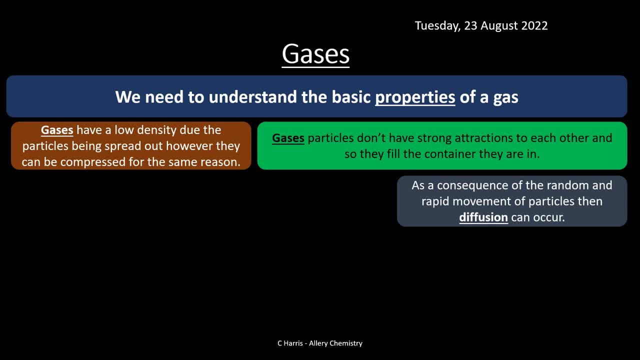 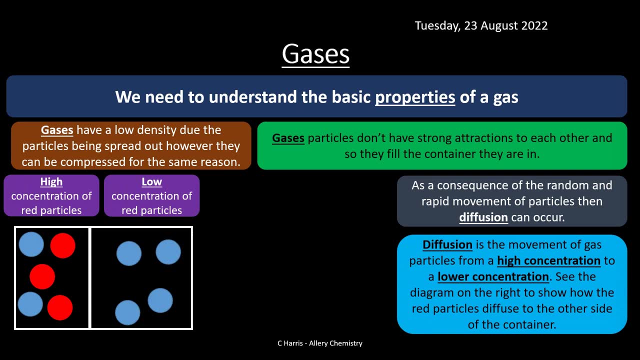 Now, if you're a biologist, you've probably seen this quite a lot With cells et cetera, And this is obviously no different. There's no difference within chemistry, But diffusion is affected with the movement of gas particles from a high concentration to a lower concentration. 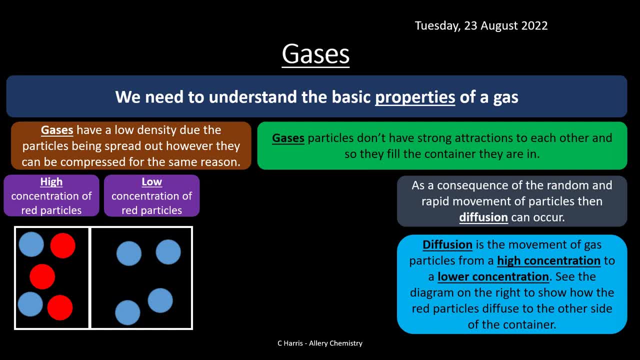 And obviously, if we look at this diagram on the left here and we can see in terms of the concentration, our substance of interest is the red particles here. So you can see obviously high concentration on the left. As you can see, there's loads on there. 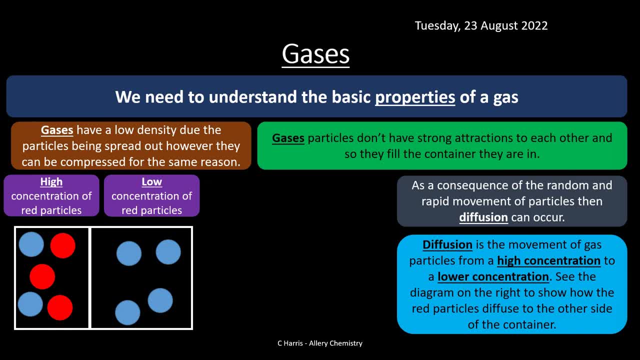 And there's a partitioning line And on the right-hand side you've got a low concentration of particles there And hopefully you can see that there. So obviously diffusion is the phenomenon where when we mix them, say, if we open that partition up, then the particles will move from a high concentration to a lower concentration. 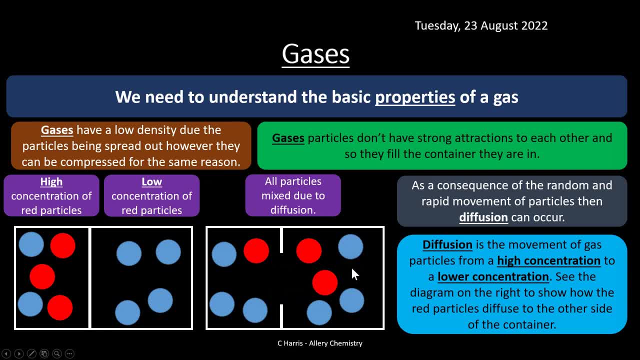 And obviously that will kind of diffuse across. And this is quite a unique property, fairly unique. I mean liquids can do it as well, But gases have this ability to kind of mix quite well And diffusion can occur in gases. OK, so now we're going to look at something called ideal gases. 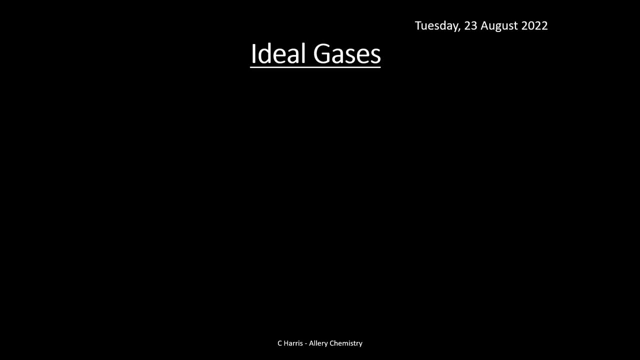 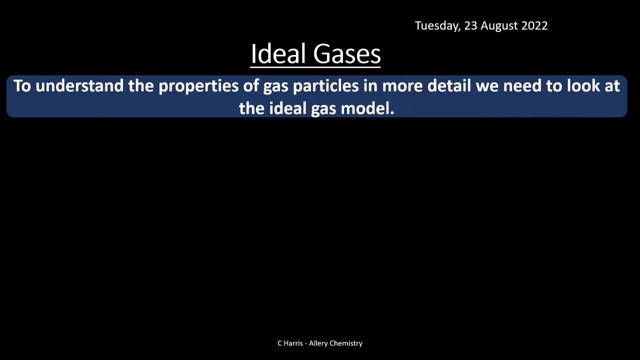 Now it sounds quite, I don't know, sounds very surreal. I think is a bit weird. It's like: well, how can you have a gas? that's ideal, But you can. So here we are. So, to understand the properties of gas particles, we're going to look at something called an ideal gas molecule. 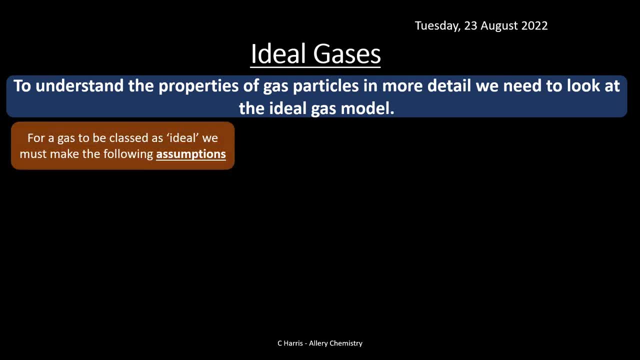 Ideal gas model, should I say- And this gets a little bit weird, a little bit complicated. But for gas to be classed as ideal, ideal, we must make these assumptions. now, don't worry too much about these. it's just kind of talking about, you know, the kind of properties of gas. it builds up into an equation which we'll see. 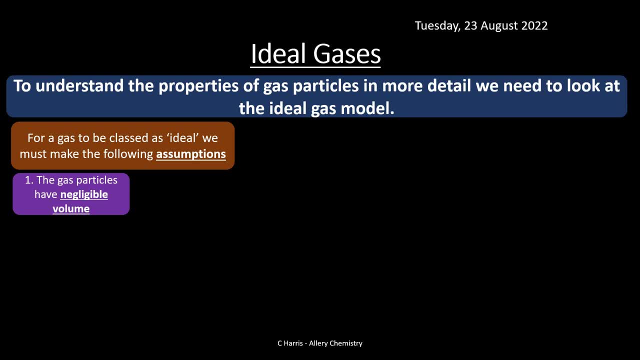 later, which you really do need to know. um, so gas particles have negligible volume. okay, so, um, they obviously don't have, um they don't have, you know, any kind of um, they don't occupy a large, large space, basically, and you know the volume is quite small. um, the gas particles are equally sized, they. 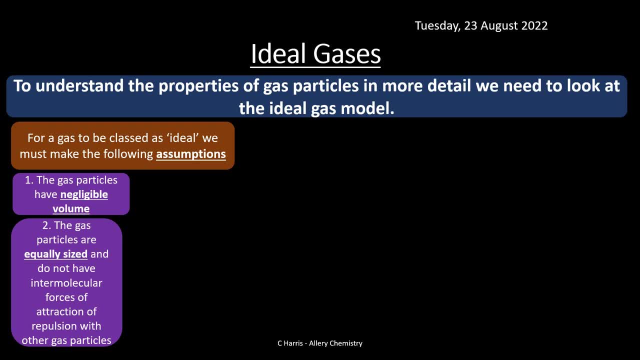 don't have any intermolecular forces of attraction. you would have seen that in topic three, um of repulsion with other gas particles. so that's what we assume. if something is ideal, the gas particles will move completely randomly and continuously, ie they don't stop and the gas particles have. 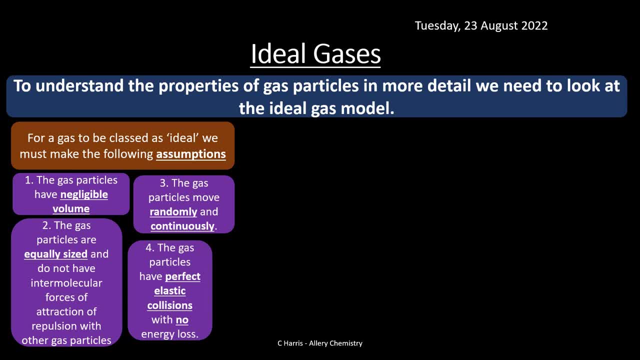 perfect elastic collisions with no energy loss. now, for the physicists out there, they'll probably know exactly what that means. but for the non-physicists? basically, if you have a collision that is perfectly elastic, um, there is no energy loss whatsoever. now, in reality, when you collide things together, there is energy loss. so it's either heat, it could be sound, it. 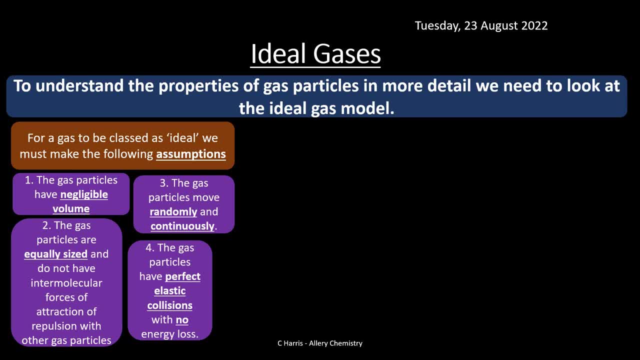 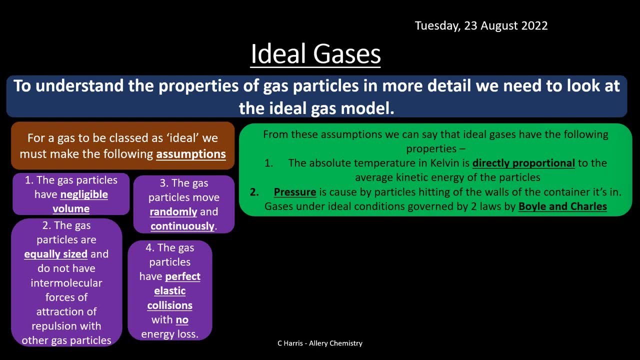 could be light, it could be various different forms of energy. um, in an ideal gas. we assume that this doesn't happen. okay, something that's ideal. so from these assumptions we can then say that ideal gases have the following properties. so, um the absolute temperature, um in kelvin, is directly proportional to the average kinetic energy of the particles. okay, 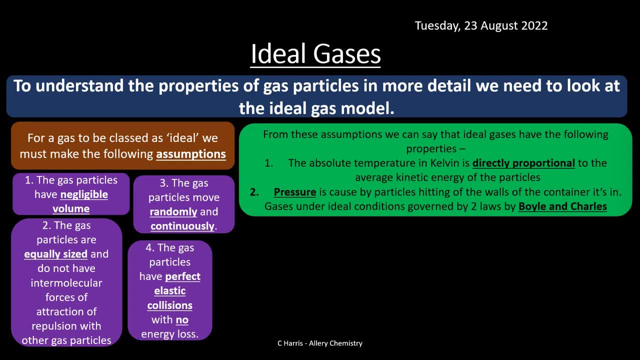 that's what we can kind of say, um. and then pressure is caused by particles hidden off the side of the walls of the container it's in. so gases, under ideal conditions, are governed by two laws. and you've got boyle and you've got charles. okay, these two, um, i suppose, scientists, physicists. 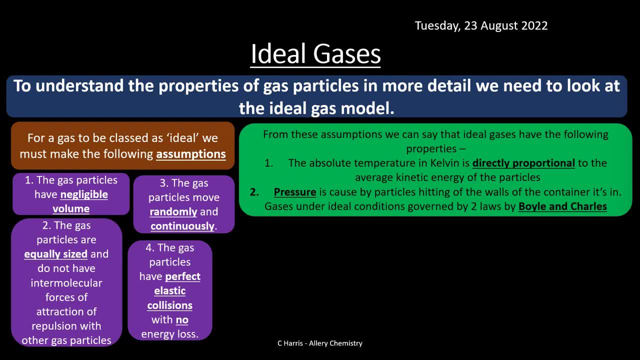 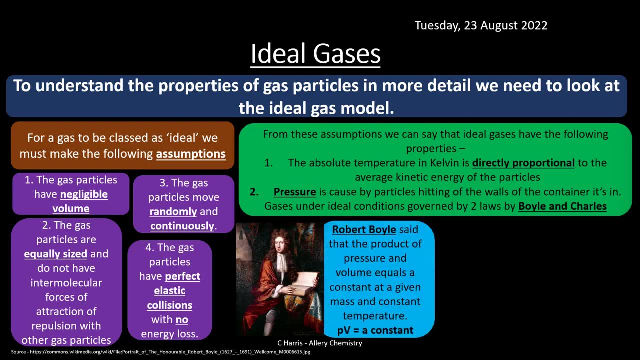 probably more likely to be um, these two scientists um came up with two laws um about gases, and they loved gases. if you, if you, really hate them, these people loved gases. so robert boyle was the first chap and he said that the product of pressure and volume equals. 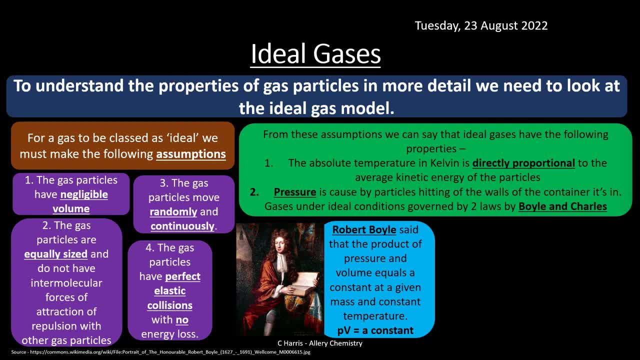 a constant at a given mass and a constant temperature. so he said pv, which is the pressure and volume, equals a constant. okay, so basically he said there was some correlation there between the two. again, don't worry, you don't need to know the kind of ins and outs of this, it's just kind of. 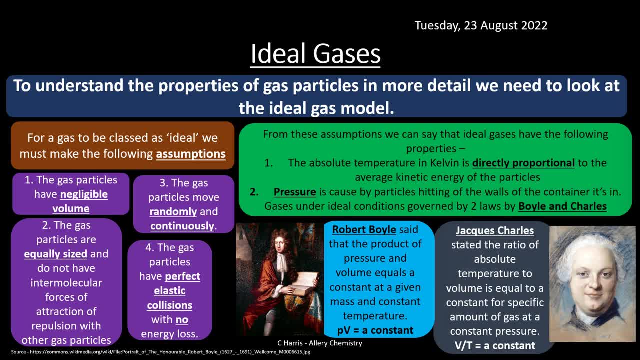 setting the scene. i suppose, uh, the second uh chap was jacques charles, who was a french- uh, i think, believe he was french. yes, he was a french scientist- and he stated that the ratio of absolute temperature to volume is equal to a constant for specific amount of gas at a constant temperature. so he said that um v over t. 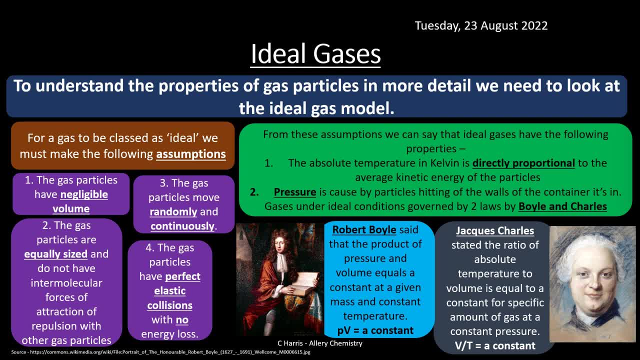 equals some form of constant. so these two people had these kind of ideas and, like in science, a lot of scientists will collaborate with each other and they're going to collaborate with each other and kind of nick each other's ideas and use their ideas and be inspired by them. and this was like the 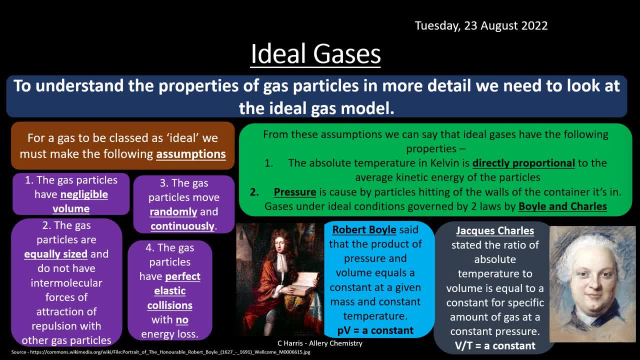 big thing back in the day of these. these two chaps kind of existed a few hundred years ago and but for them it was, you know, they were like kind of the pop stars of the day and they basically came up with these two theories and actually if we combine them together we can actually come up. 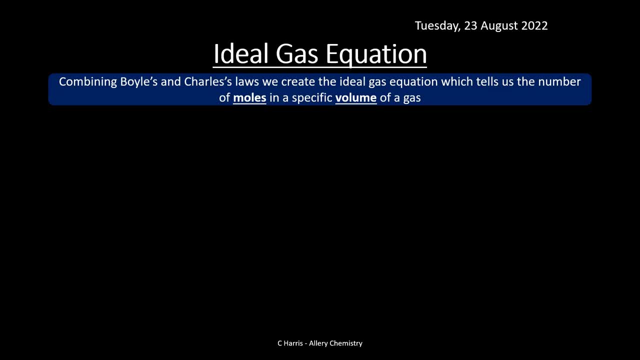 with something called an ideal gas equation. so we talked about what an ideal gas would look like or how an ideal gas would behave, and we talked about what an ideal gas would look like and we talked about how an ideal gas would behave. and we talked about what an ideal gas would behave and we talked about. 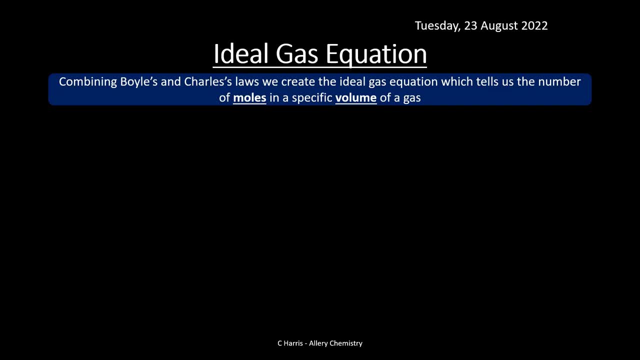 in reality, obviously, that doesn't really exist, does it? you know these ideal gases? but it's a, it's a, it's a theory, it's saying right, we can have gases which are more ideal than others and we can look at the properties of them and you'll see you. you will have to use the equation for this as well. 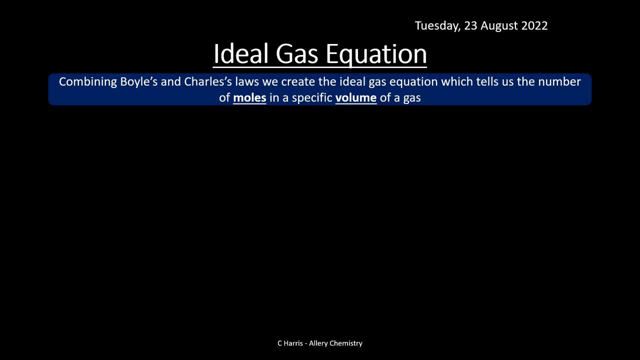 and, but basically it tells us um the number of moles in a specific volume of gas, which is quite useful because gases are obviously an important part of chemistry, and they basically mash the two equations together, and this is the one you do need to know. this is the ideal gas equation. 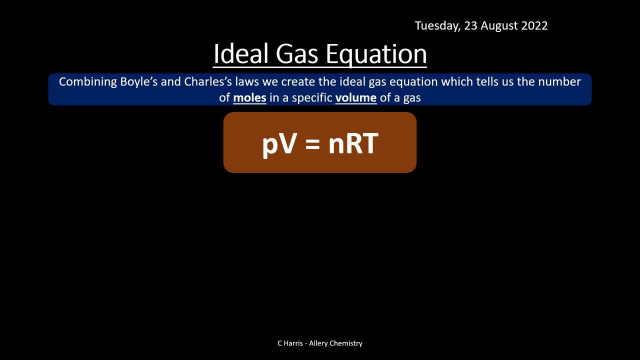 p. v equals n, r, t. okay, so p is the pressure in pascals, v is the volume in meters cubed, n is the number of moles, r is a gas constant. so remember them. two chaps came up with the constant. we've actually put a number to it this time, which is 8.31 joules per kelvin per mole, and t is the. 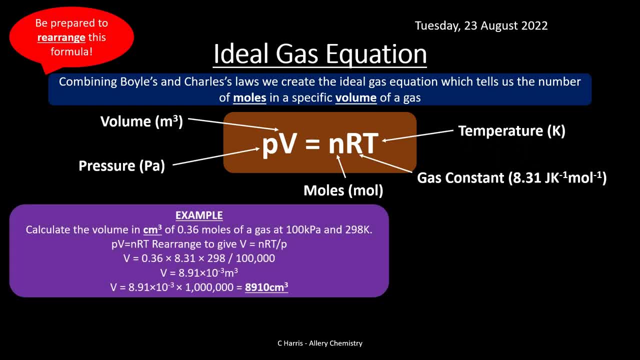 temperature of the gas that we're looking at. so we need to be able to use this equation and we have to be able to rearrange it, and we have to be able to obviously use the equation here as well. so let's look at an example. so we're going to calculate the volume in centimeters cubed of 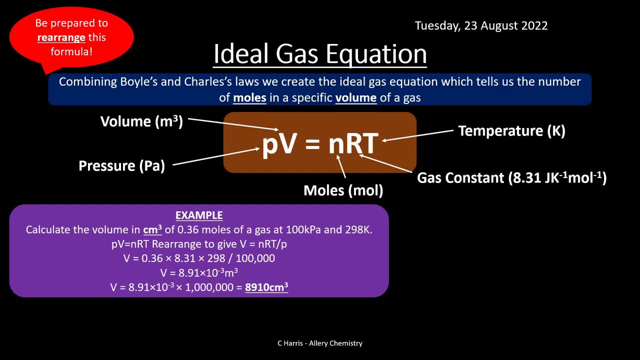 0.36 moles of a gas at 100 kilopascals and 298 kelvin. now pb equals nrt can be rearranged to give v equals nrt over p. okay, now one of the key things here. I'm going to point out some key things. 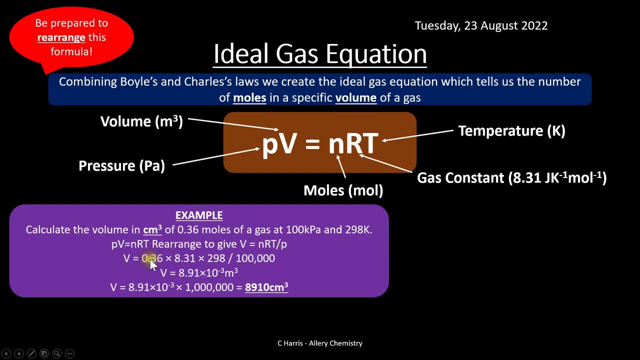 as we go through these numbers here. so obviously the n bit is the number of moles, which is 0.36 moles. fine, so we know that 8.31 is the gas constant. that's always going to be the same. that isn't going to change in this example, unless the exam. 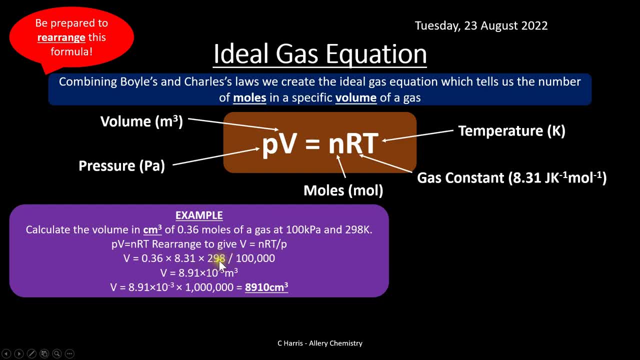 board gives you something different, but you know that's always the same. 298 is the temperature in kelvin, which is here, and we're going to divide that by the pressure. now the pressure is 100 kilopascals. remember, though, the unit has got to be in a number of moles, so we're going to divide that. 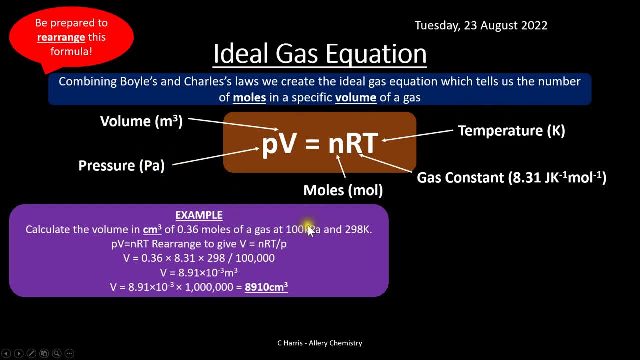 by the pressure. and when we do do this, we always want to use factor of a thousand because, um how you convert from centimeters cubed to meters cubed, to decimeters cubed? if you're not familiar, you're not comfortable with converting units, make sure you go back and have a look at. 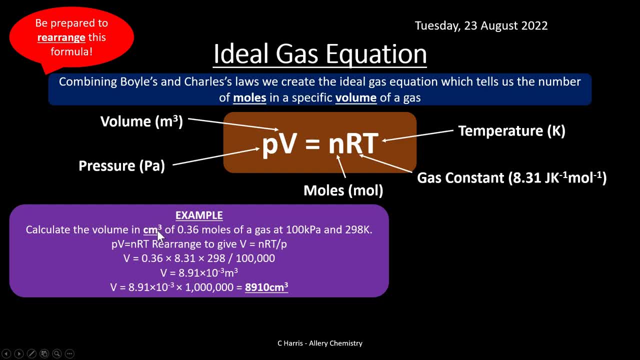 our video for topic two. it's really, really important. so it's when we looked at the mole calculations and things like that. so anyway, so the to convert from meters cubed to centimeters cubed, we need to multiply by a million to get that. so we take 8.91 times by 10 to the minus. 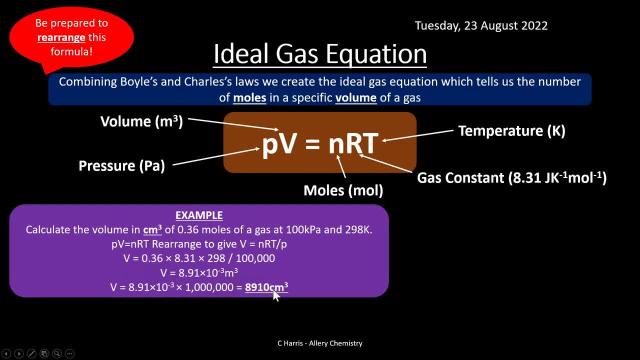 three, multiply by a million and we get 8910 centimeters cubed. so the volume of this gas, 0.36 moles of this gas, at this pressure and temperature, would occupy that much space. that's basically what this equation is looking at. so, um, the next slide i've- i've removed it from this, just. 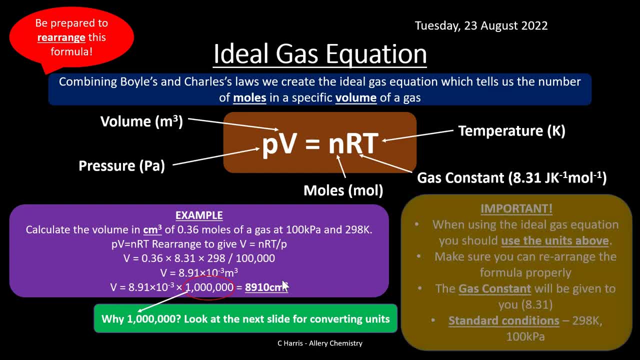 to kind of keep it simpler. like i say, look at topic two for that um as well, so important. so when you're using the ideal gas equation, you should use the units above. it's really important, as i mentioned before. make sure you can rearrange that formula as well. you've got to be familiar with that. the best thing to do with. 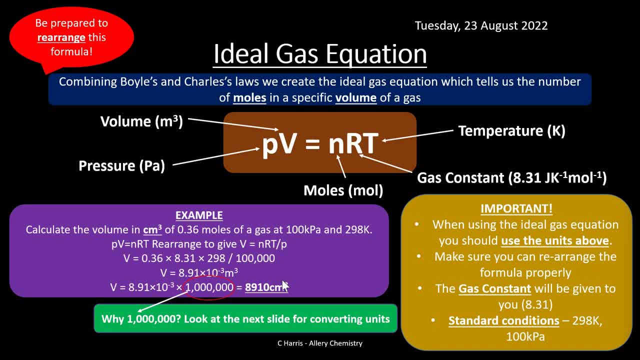 these is to again practice. a lot of this is maths related and there's some equations here. it can get very boring if i'm sitting here just working through loads of different examples. but work through it, have loads of exam questions and practice them until you literally go blue in the 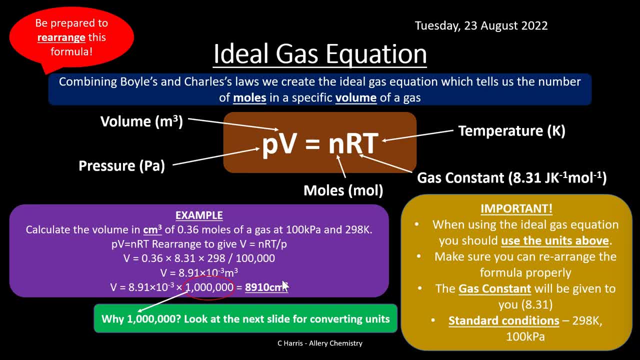 face. well, not literally, because that would be quite dangerous, but you know what i mean. um. so the gas constant will be given to you. it's 8.31 joules per kelvin per mole, unless they give you something different. but i don't think they will be 8.31. um, and standard conditions is obviously 298 kelvin and 100. 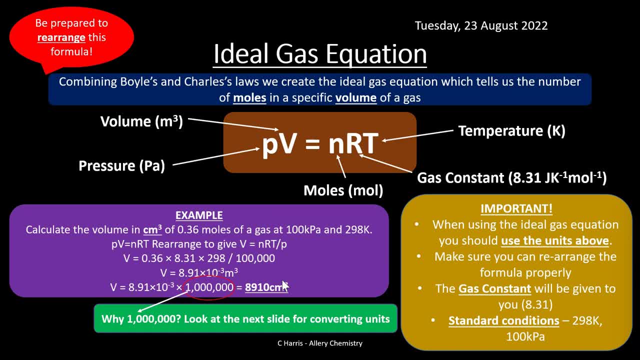 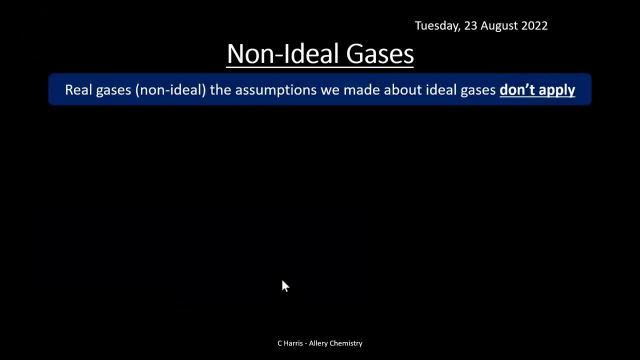 kilopascals of pressure. okay, so right. so let's look at some non-ideal gases then. so we've looked at some ideal ones. now let's have a look at some non-ones, so real gases which are just like you know what, like everyday gases. i suppose they're classed as non-ideal in reality. 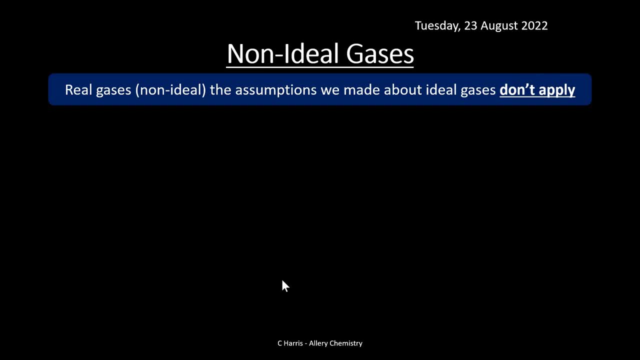 ideal gases don't really exist, but that we have a kind of theory to show an extreme and then we can measure something against that. so that's why that that equation is important. but real gases are non-ideal. the assumptions we made obviously don't apply. so when we increase the pressure of a gas, 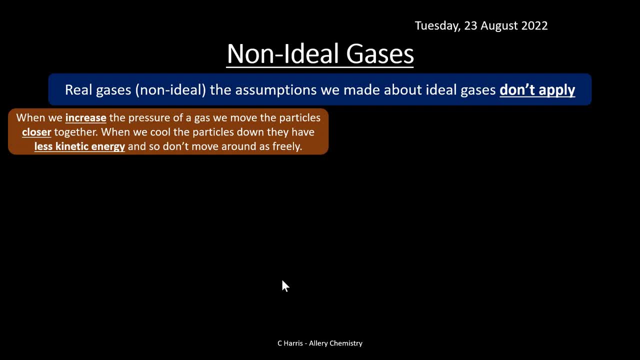 we move the particles closer together, don't we? so when, when we heat, when we increase the pressure, we're squashing them together. and when we cool the particles down, they have less kinetic energy, so they don't move around as freely. okay, so obviously that does exist in reality. and also if we look at this diagram here, we can see: 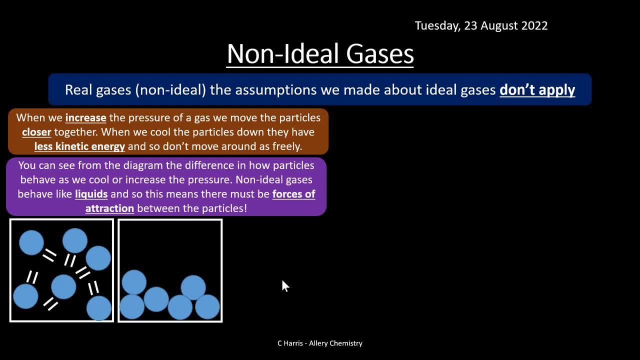 the difference in how particles behave as we cool or as we increase um the pressure and non-ideal gases do actually behave like liquids, um, to an extent. so this means there must be forces of attraction between the particles. so, for example, um you might have seen it, i'm not sure you you. 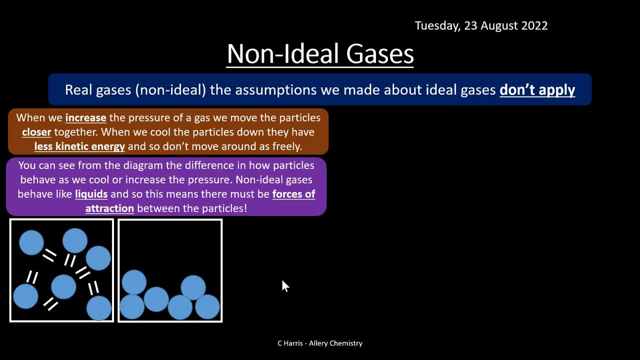 might have done. actually, if you look at something like liquid nitrogen or or maybe even liquid, you can actually pour it out when it's really cold and you'll see it kind of flow, flow outwards and it looks like a liquid's been poured. so for that to happen, there's got to be forces between these. 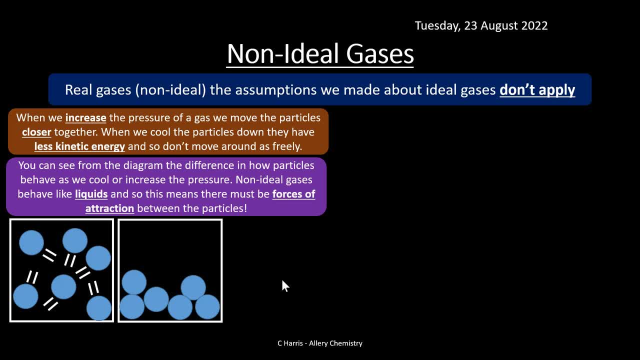 particles. now the ideal gas um scenario. assume that there aren't any forces between these, which doesn't really exist, does it so? so yeah, so this is kind of showing you the difference here. obviously it does behave like a liquid. when we cool it down, it kind of clumps together. here they have less. 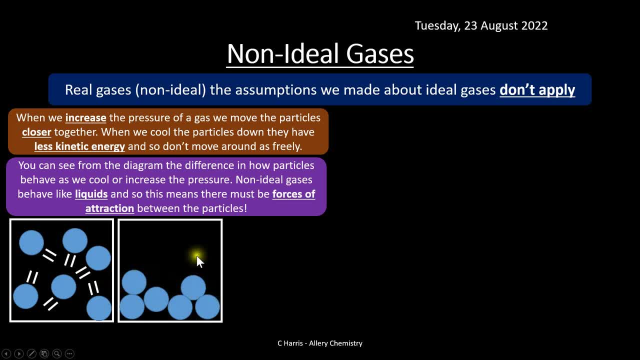 energy. they're a bit more lethargic and they kind of just collect a little bit of energy and then at the bottom, if you tip that box over, you obviously get liquid. you know behaves like liquid, it can be poured. so obviously the particles take less space as well, and obviously that didn't. 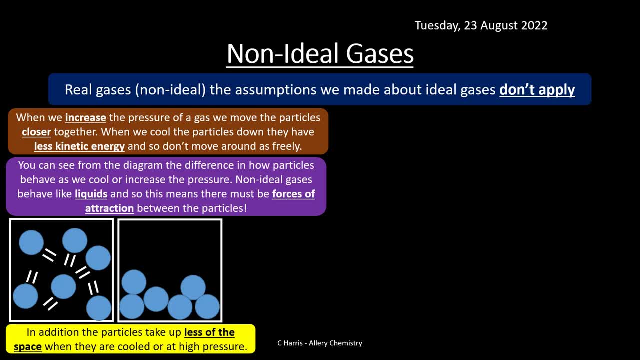 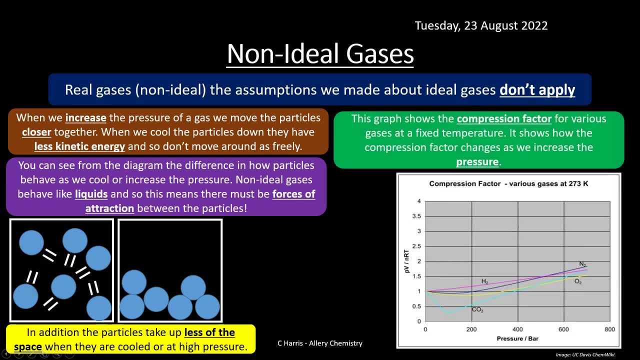 fit with the ideal gas theory. um, so obviously they're not taking as much space as, say, a normal gas profile like this. okay, so just kind of put this in graph form then, because the exam board again, you don't really need to be too fussed about this, it's just the exam board might give you. 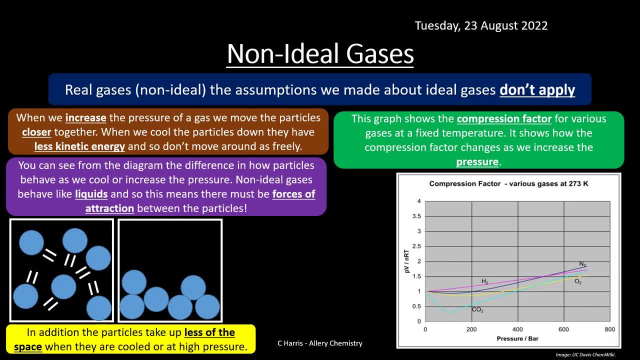 graphs like this and you might think: well, what's it talking about? and it's just kind of giving you some ideas of how the they could expand on this, to use a pun. um, so this graph basically shows something called the compression factor. so if we're squashing gases and we're squashing various 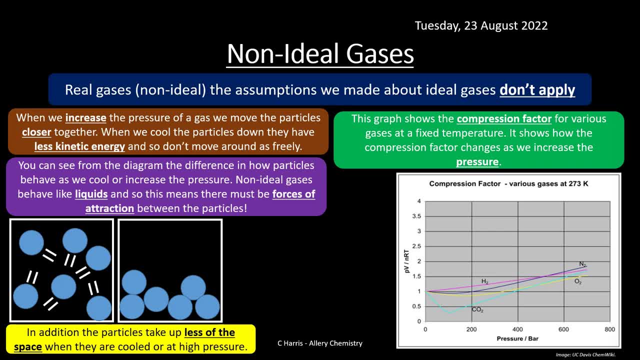 different gases at a fixed temperature and it's basically going to show what the compression factor is as we increase the pressure. so how that changes, how does the the factor of compression for these gases changes as we as we change the pressure on it. so you can see an ideal gas. 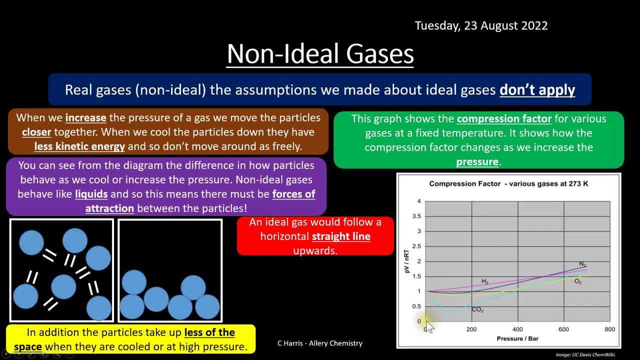 really would follow a horizontal straight line upwards, so it'd start from here and just work its way upwards directly, you know, as a diagonal line. now you can probably see some of these gases. clearly don't follow this profile. and look at carbon dioxide when we increase the pressure. 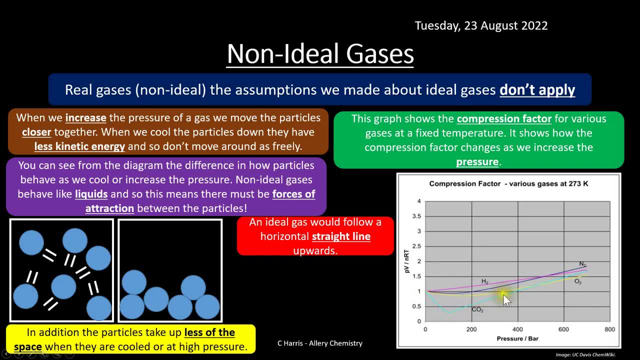 the compression factor actually decreases and then it starts to increase. you know, when, following a kind of typical ideal profile- hydrogen, as you can probably see here, there we are- hydrogen obviously follows probably a closer to the ideal profile. if we're thinking about the carbon dioxide, as we're, 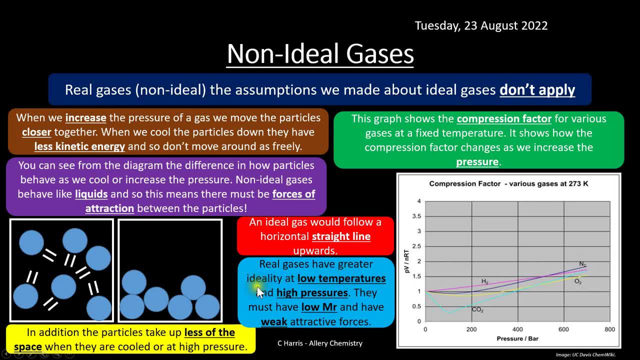 profile to that. but real gases actually have greater ideality at low temperatures and high pressures. so you can see here the back end of these graphs. here they're kind of more of a diagonal profile rather than at the start. some of these are curving at lower pressures. 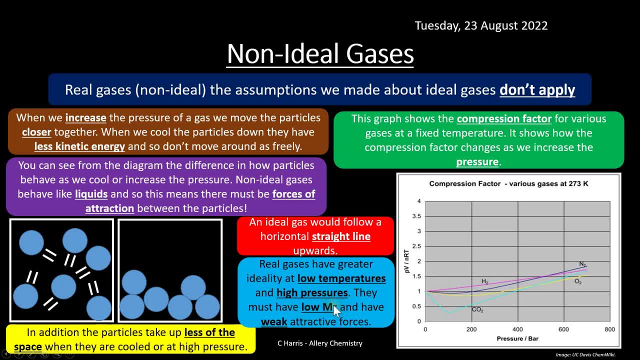 so um, and they must have. for them to kind of follow this ideality, they must have a low molecular mass as well. so lighter the gas, the better, the more well, more closely it's going to follow an ideal profile. and they must have weak attractive forces as well, so anything with a bit of polarity in like. 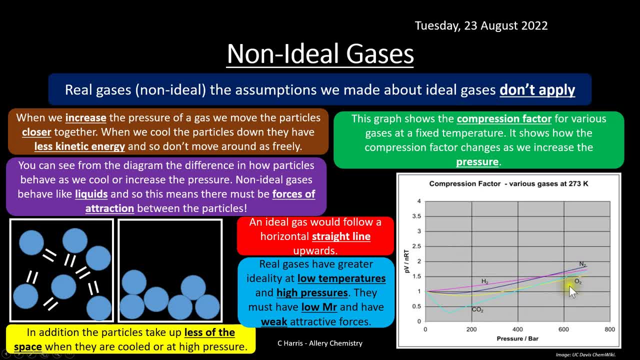 um, you know, for example, oxygen might have van der waals between it, and nitrogen will as well, carbon dioxide will as well, though it's classed as non-polar molecule, but it can have van der waals forces as well. so you know, these forces can exist. so if we look here, basically hydrogen. 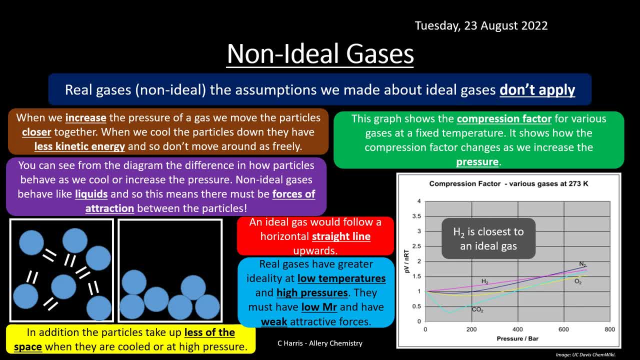 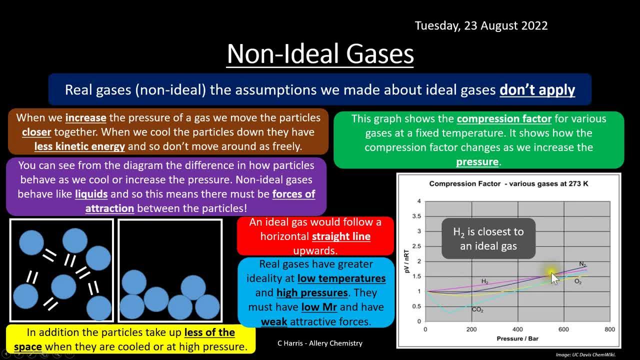 deviate too much. and it's going to deviate too much and the lower pressures, and it just follow that classic kind of diagonal, um kind of line there. so it's the lightest one as well. so it's just kind of going through the difference between ideal and non-ideal gases. okay, so let's move on. 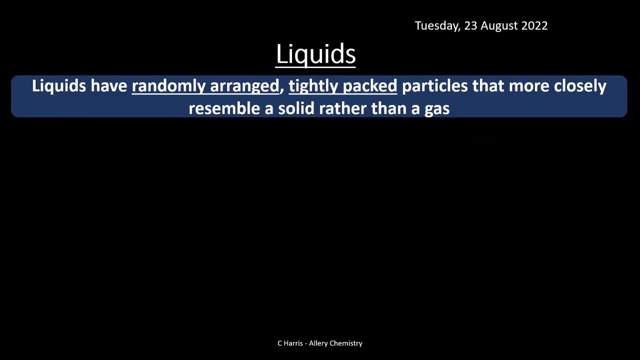 let's look at liquids then. so obviously, we looked at gases, and that's what you need to know about gases really. uh, liquids, they are randomly arranged, as we've seen before. they are tightly packed together- um, you know much more than gases, of course- um, and they actually kind of resemble. 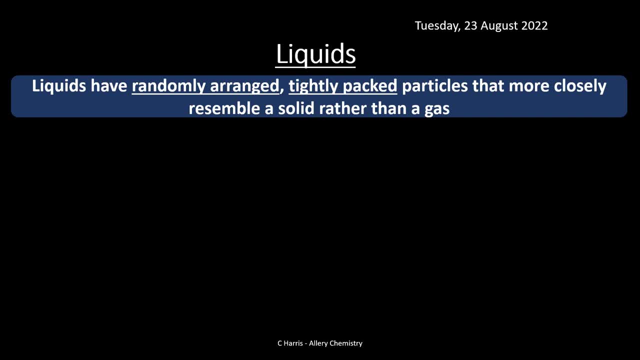 more of a solid than than a gas. again, if you use a syringe and put your thumb against the syringe and fill that with a liquid and try and push the syringe, you're gonna, you're not going to compress that. you know that syringe, the plunger is not going to kind of dip any further because the 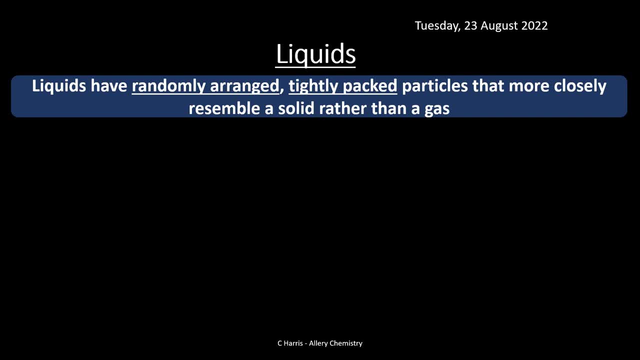 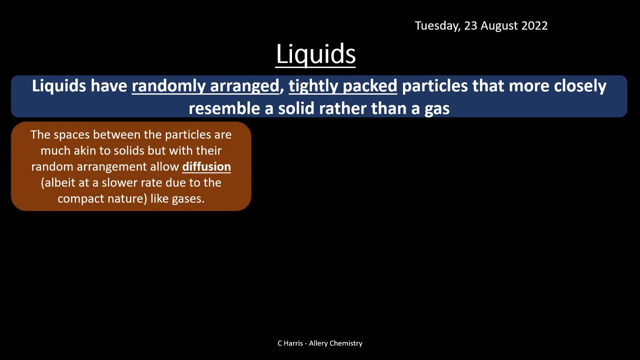 liquid is quite tightly packed, whereas if you did that with the gas it would compress. so, um, looking at liquid then. so the spaces between the particles are much akin to solids, um, but their random arrangement do allow diffusion to happen. so if you're looking at a liquid and you're looking at 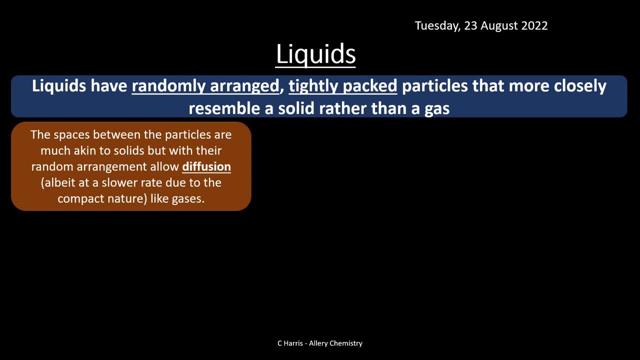 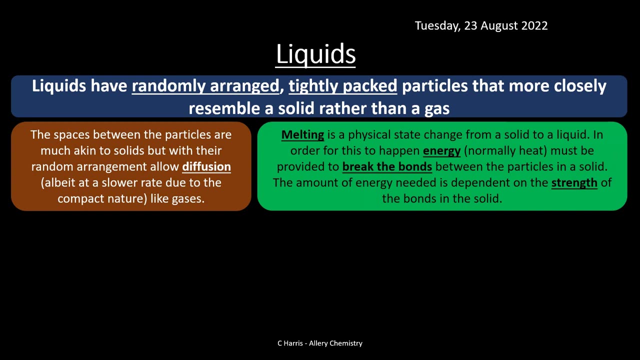 just like you do with gases. so they're kind of a bit of properties of gases and a bit with um, with solids as well. um, although they do kind of diffuse at a slower rate because they are a little bit more compact, it's, they're not quite as kind of free to move around like gases are, so melting um is a. 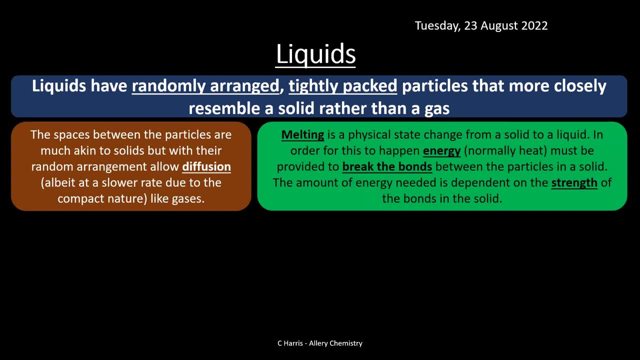 physical state change from a solid to a liquid. obviously you would have seen that. so in order for this to happen, obviously you've got to put heat energy, and it's normally heat, you know, in the universe, and there's a lot of energy in each part of it. but, understandably, говорю. 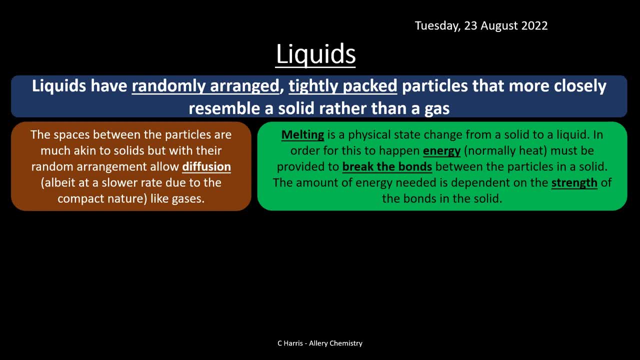 so in terms of natural causes of energy and all of these really relate a lot actually to the physical properties, and so there might have been anti joka sometimes and there might be something with so-called microgravity, and this might be a very small particle there. but if, if you were to, 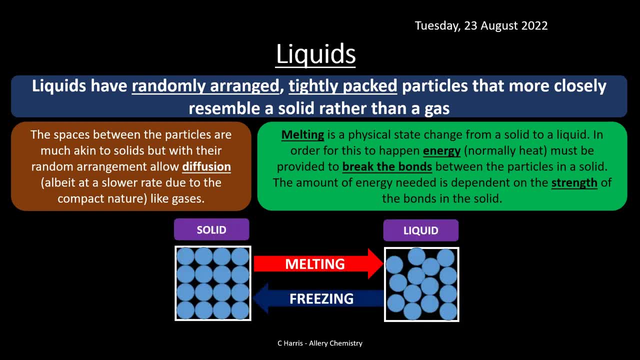 explain why it's shocked. you know sarca knot or anything. so, basically, you know we could have lived in방en days of trajectories, particularly if we were talking with ISISанием. these are the very problems you're going through. so our first fallmy second, you'd think, hey, what's all this? 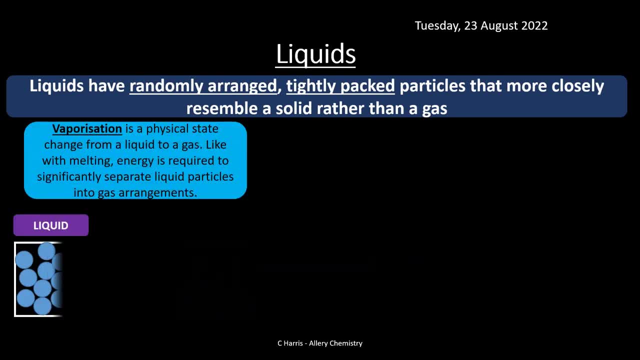 which is obviously freezing. so um kind of going the other way, um obviously going liquid to gas. this is called vaporization and it's a physical state change. um and obviously, like with um melting, energy is required to um obviously separate the particles of the liquid to turn it into a gas. 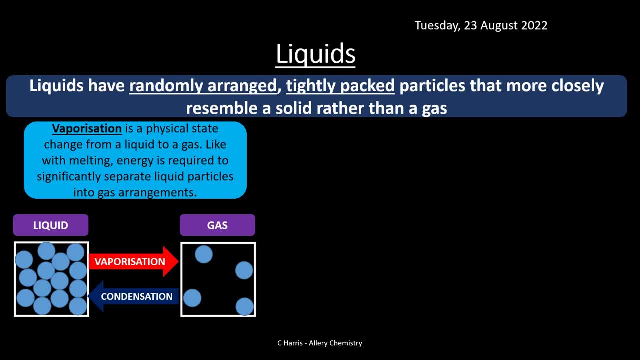 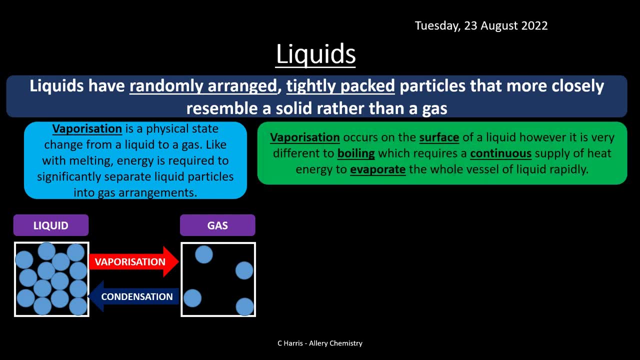 vaporization is the term that's used to move it from a liquid to a gas, and going from gas to liquid is condensation, a bit like what you get in your windows. so vaporization occurs on the surface of a liquid. um, it's very different to boiling, though, so just be really careful, okay, so um you. 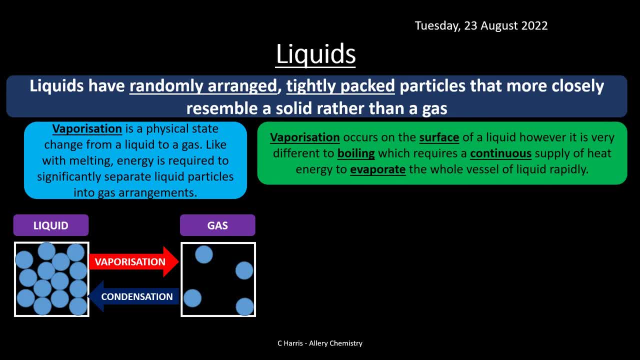 know, water can evaporate into the atmosphere, but it doesn't need to be boiling to do that. obviously. we see that you know everyday life, don't we? when it rains, um, and you get water on the pavement, let's say: then, when the sun comes out, it evaporates, but it's certainly not boiling, because we wouldn't. 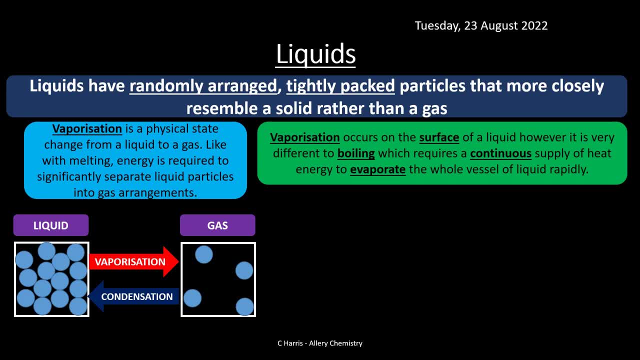 survive. so you don't need boiling temperatures to turn a liquid into, such as water, for example, into a gas. you don't need that, okay, so that's that's what i want, to get that distinct difference out the way. okay, it doesn't have to be a boiling point for vaporization to occur. okay, um so, but it. 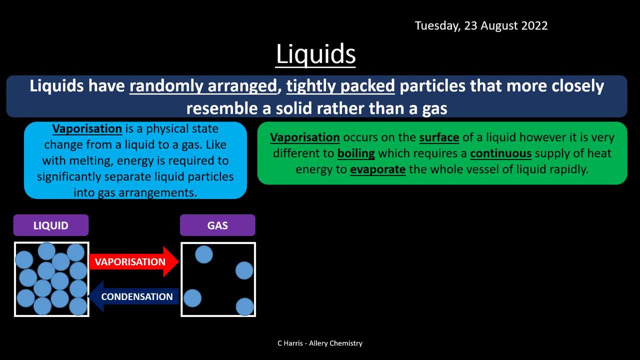 doesn't require a continuous supply of heat energy to evaporate it, though. okay. so that's that's, you know, really important. so if you had a big, you know vat of liquid, for example, and you want to get rid of that as quickly as you possibly can and you really do want to apply an extreme amount of 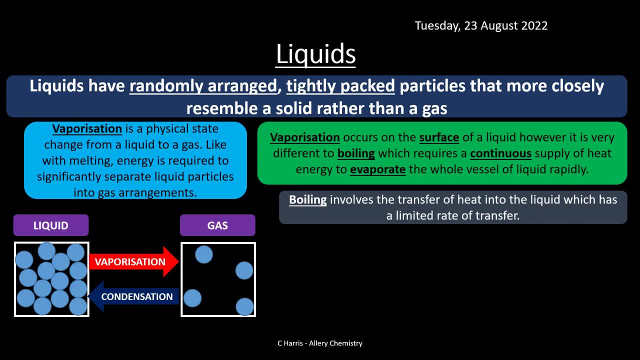 heat to that to get evaporating quite quickly. so evaporation happens at the surface of the liquid. okay, so boiling involves the difference between vaporization and boiling is boiling involves the heat into the liquid, which has a limited rate of transfer. so if you imagine a pan of boiling water, 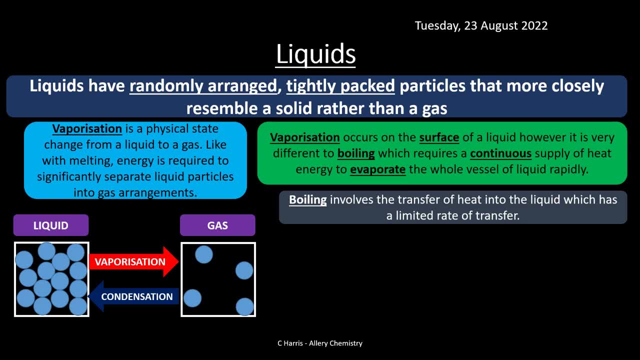 um, you boil the pan, um, you get water vapor at the top of the water. don't you say they get that? but there's actually heat energy within the main body of the water and that's because you can see the bubbles, can't you see the particles kind of moving around like that? so, but obviously the rate. 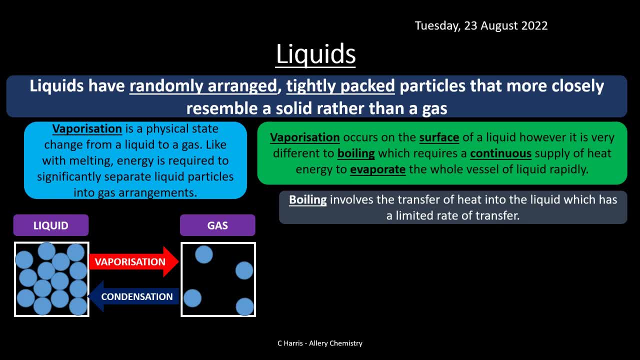 of transfer and sometimes this can happen. actually, if you've ever done it with soup in the in the microwave, it spits quite a lot. there's a lot of kind of what we call bumping, and basically some of the energy that's within the main body of the liquid builds up and it spits out of spits. the. 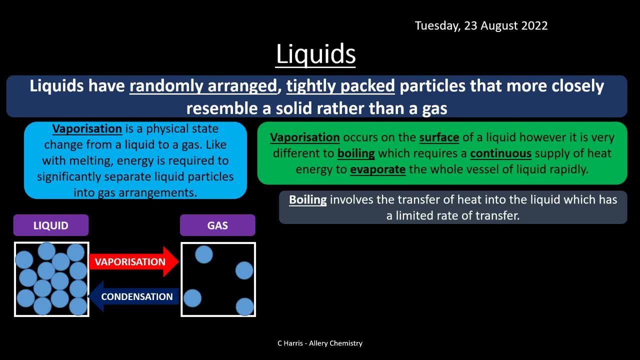 actual liquid out of the pot, so, um, and obviously the reason why it's doing that is because it's just taken too long for the energy to escape from that liquid through vaporization, so instead it just jumps out of the pan instead, or the bowl, so, um, and that's basically where you've got something. 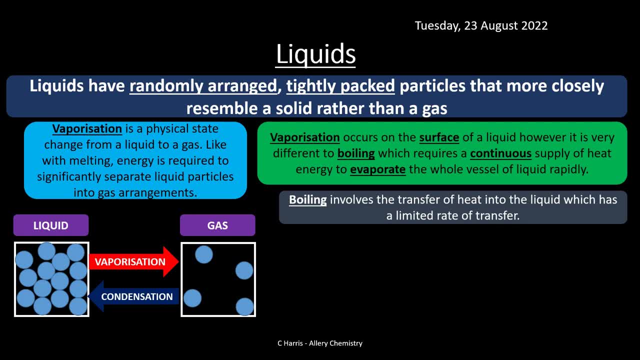 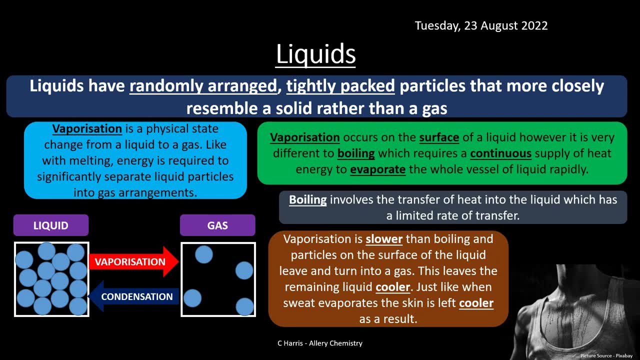 that's boiling. something will boil if the rate of vaporization is not quick enough to get rid of the energy that you're putting in. that's basically what boiling is okay. so there we are. you've learned something new. um, so vaporization is a lot slower than boiling, as you can probably understand. um and particles on the 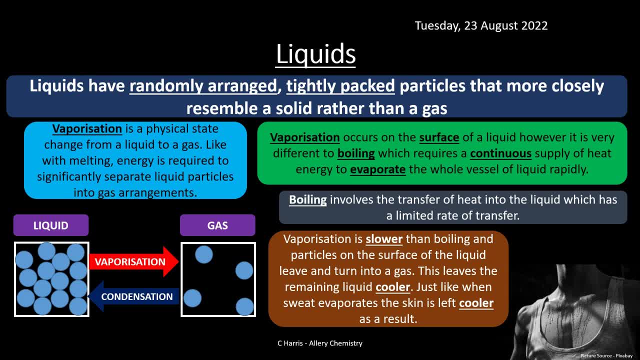 surface of the liquid leave and they turn into a gas. it's always on the surface and this leaves the remaining liquid cooler, because some of the energy that was in the liquid is now obviously being used to break the particles apart or move them further apart and turn it into a gas. 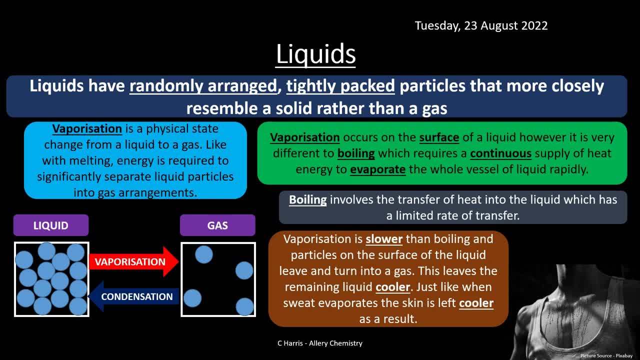 and this is effectively how, when you do exercise and you sweat, um, obviously you've got um, you know. when you're running, you're you're doing any form of physical activity, uh, or if it's just a warm day, your body temperature starts to get warmer. now your body has to try and get rid of that heat. 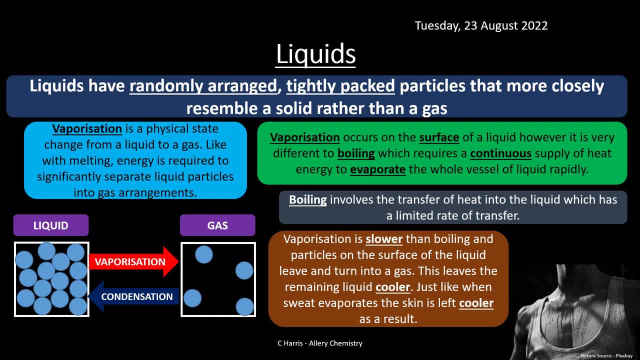 energy in some shape or form. otherwise you will. you know you you won't, you'll probably pass out with heat stroke or something. so your body produces sweat as a liquid, and what that does? that liquid coats the surface of your skin and it's designed to absorb the heat from the body. 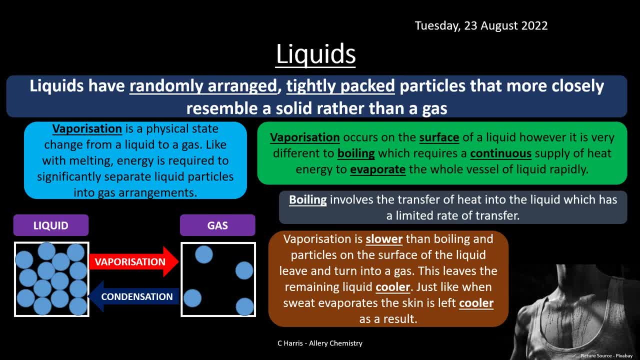 and evaporate. now, the whole point of having sweat glands all over your body, or the vast majority of the body, is to increase the rate at which that heat can be taken away from the body. and obviously, the more exercise you do or the harder you work, the hotter your body gets, the more sweat you produce. 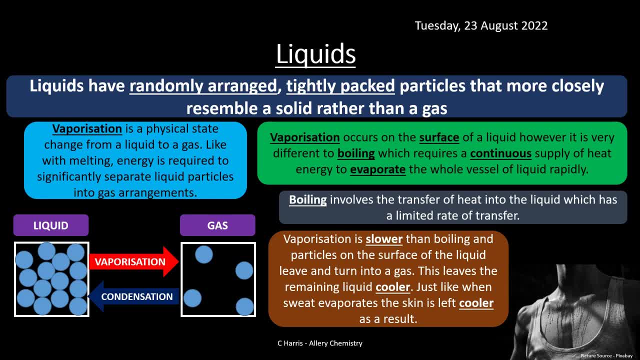 and so all of this is designed to leave the skin cooler. that's behind, because the heat energy that was in the body is in the liquid which is now evaporated out of the body. so it's a good idea to try and move some of that sweat out of the way so you can get more- you know, more- sweat, that's. 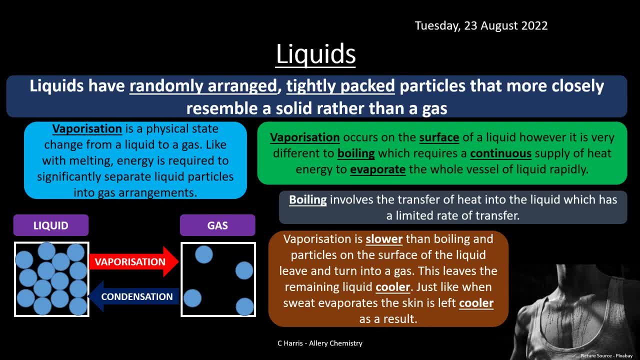 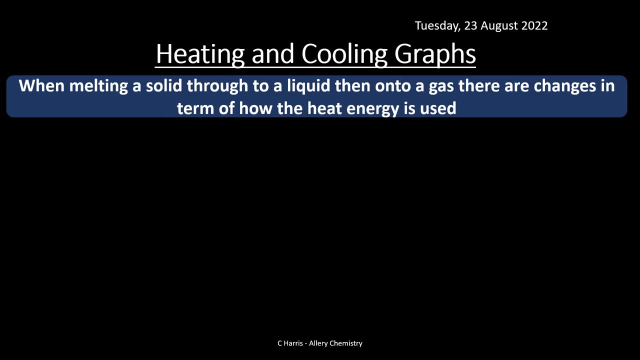 produced, and then that helps to cool the body a bit quicker. okay, so that's the difference. obviously, your body's not boiling, um, you know, it doesn't boil, but the water or the liquid does evaporate because of um vaporization. okay, so let's look at some kind of, let's look at the kind of physical. 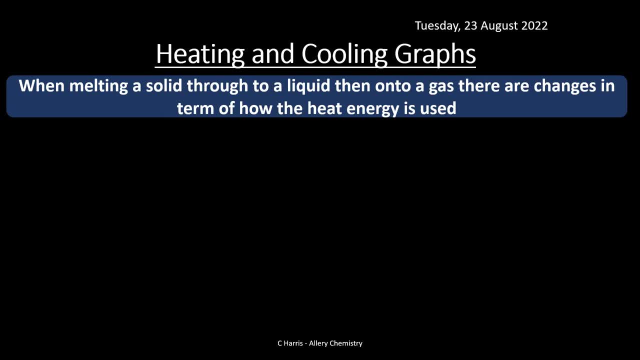 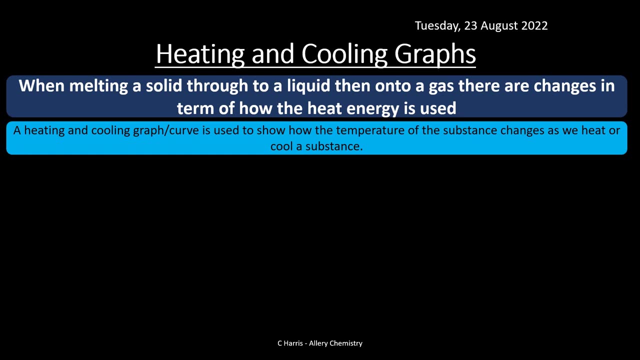 side of it. so the heating and cooling graph. so when you're melting a solid through to a liquid, there are changes in um in terms of how the heat energy is used. you need to understand what is actually happening to the particles at these different phase changes um. so we use something. 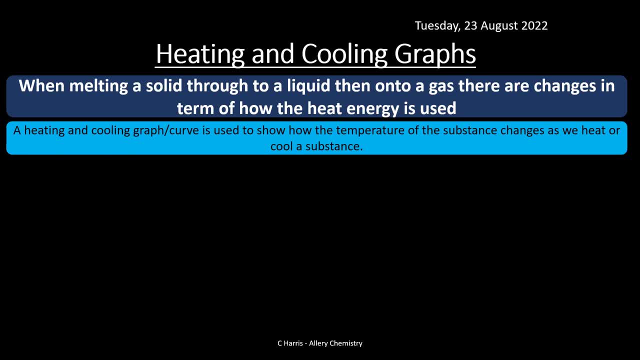 called a heating um heating cooling graph, or sometimes it's called a heating cooling curve um. it's used to show the temperature of a substance changes as we heat or cool a substance. you've got to be aware of kind of the kind of physical changes that's happened and what causes. 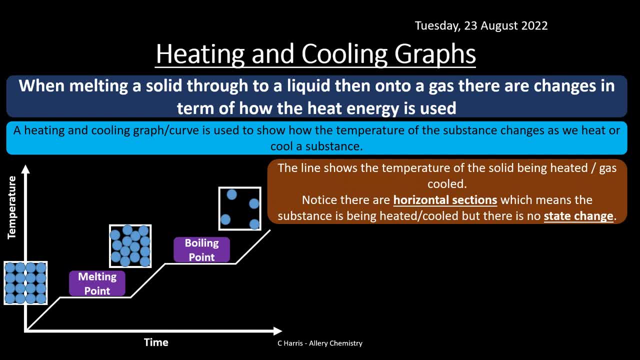 this so you can see on here the temperature of a substance changes as we heat or cool a substance. here we've got a graph here and it's showing the different um states of um. you know the states of matter. you've got your solid, which is down here at the bottom. you've got your liquids and you've 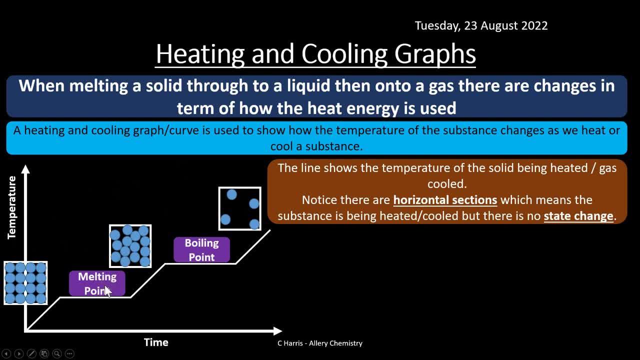 got your gases here and you've got your different um phase change points. so melting point and boiling point. so this is a heating graph. obviously we're increasing the temperature over time. the graph can go the other way and go down instead. it doesn't really make that much of a difference, they're. 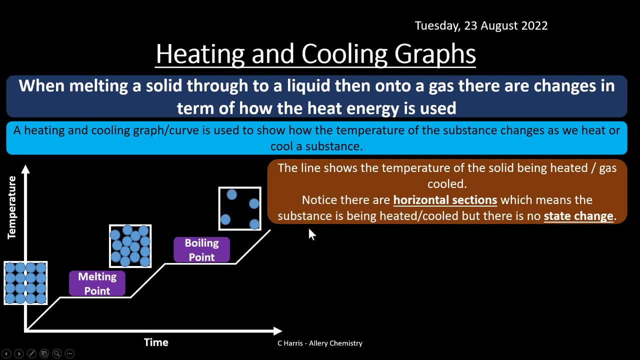 the principles the same so, but what you'll probably notice here is actually, as you heat a solid into a gas, you've got these vertical, uh so these horizontal parts of the graph here where there isn't actually an increase in temperature at some of these points, but the melting point and the boiling point you only actually get a rise in. 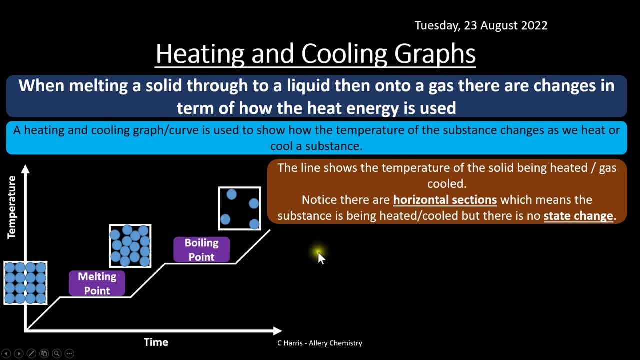 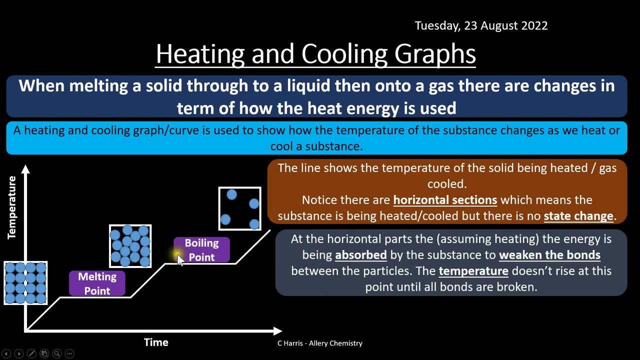 the temperature of the substance you're heating at certain points. so what's actually going on here? so if we've got, if we look at the horizontal points here, so this assumes obviously heating the energy at the bottom of the graph is actually going to increase the temperature of the substance. 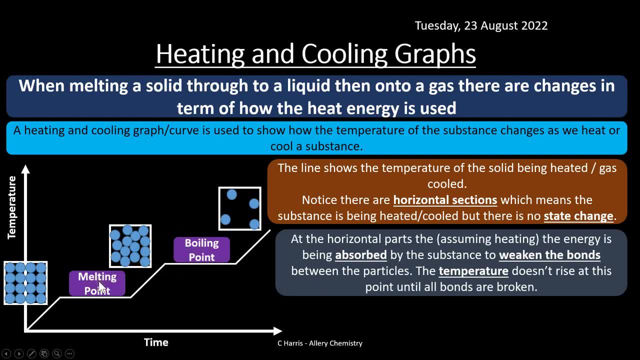 at the boiling point and at the melting point is being absorbed by the substance to weaken the bonds between the particles. so the energy that's being put in at this point- i've been putting at this point- is not actually being used to raise the temperature of the material that you're heating up. 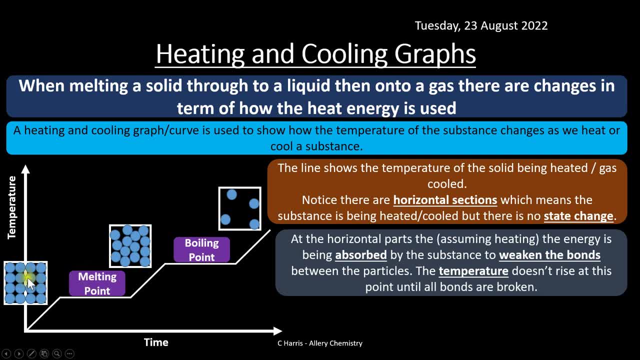 the energy is actually being used to just purely break the forces between the particles to get it into the liquid or gas state that we can see on here. so and for that reason, if you put a thermometer in your say, if you take ice, for example, and then you basically put ice in there and then you put a thermometer in, you'll notice that the 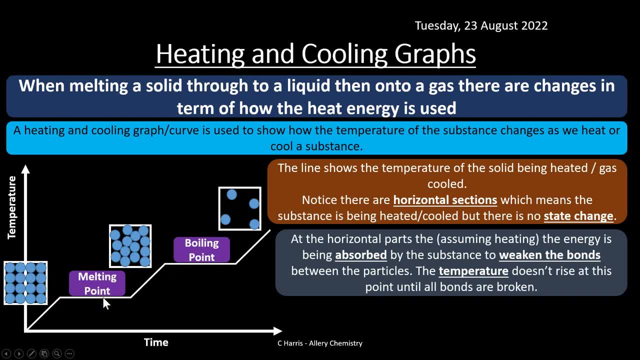 temperature doesn't change for a period of time. if you plot that kind of ice melting over time, say from obviously solid to liquid and then heated to a gas, to steam, and if you could monitor the temperature of them stages, you'll see there'll be points where the temperature just doesn't change. 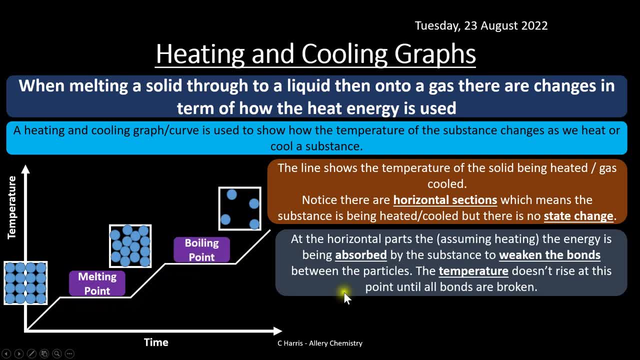 even though you're continuously heating it, you'll notice that the temperature doesn't change. it doesn't actually change. so for substance that cools, obviously we're going the other way. we're just releasing energy, as bonds are actually being formed between particles. so we'll just kind of 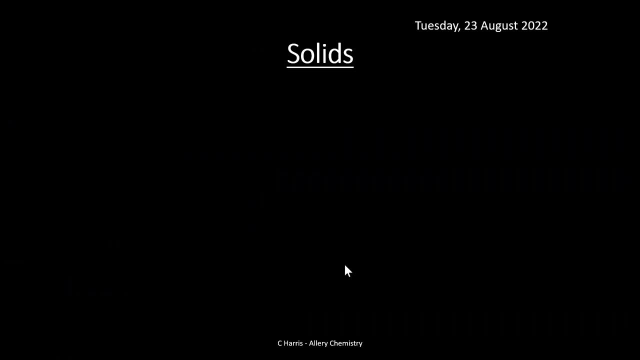 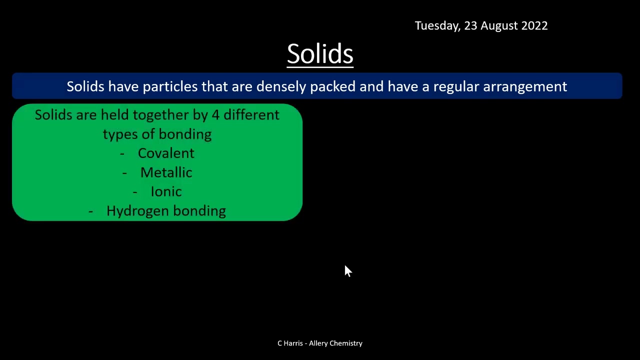 reverse it and flip it around the other way. okay, so let's look at the, the kind of the. the other state change, which is obviously solid, so the final state, so solids. obviously these are particles that are densely packed together. they do have a regular arrangement, as we've, as we've seen before. 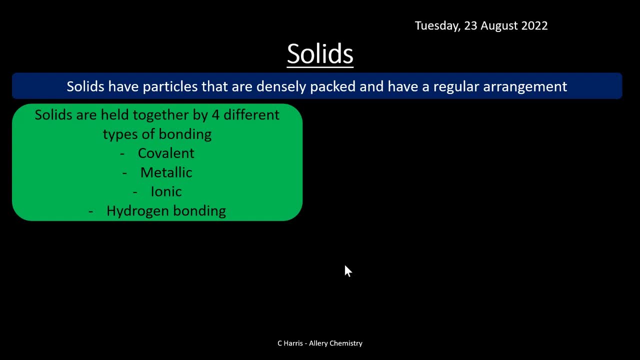 and solids are held together by four different types of bonding, as you've seen in topic three. so you've got covalent, you've got metallic, you've got ionic and you've got hydrogen. bonding is a type of force. it's not strictly really a bond technically, but it's. it's a type of force. it's. 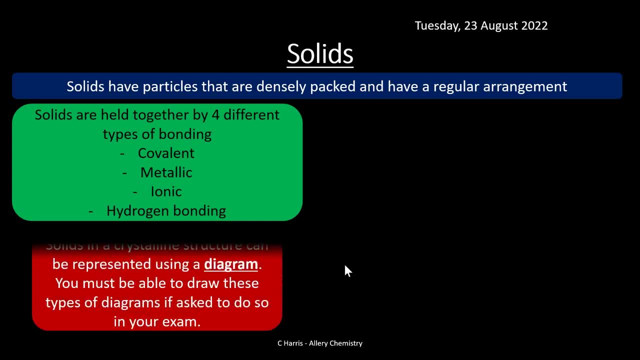 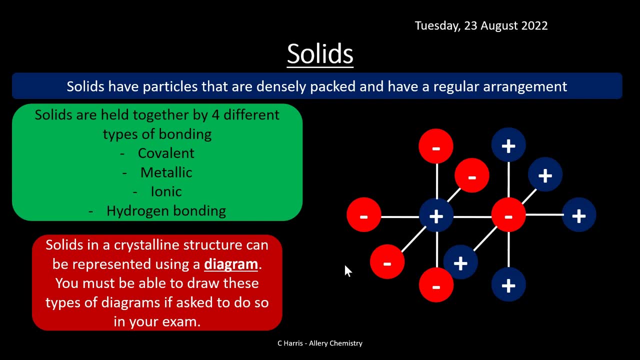 a very strong type of force. that's why i've kind of included it in here. so solids in a crystalline structure can be represented, obviously, using a diagram. again, you might have seen bits of this in topic three, and you've got to be able to draw these types of diagrams, though it's really 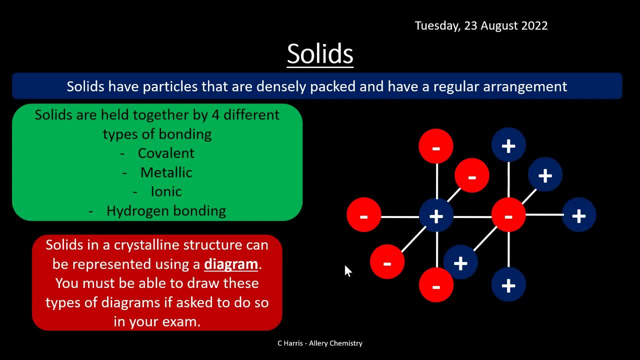 important. so you can see that, obviously, solids, you have a positive and then you have negatives that are around them and negatives surrounded by positives. so it's really important that they are regularly have a regular arrangement, a kind of structured. you can see these kind of lines and 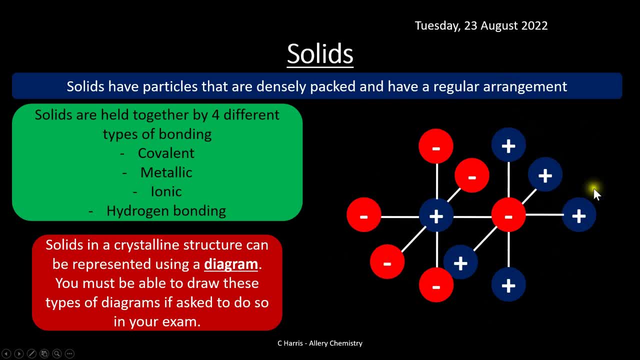 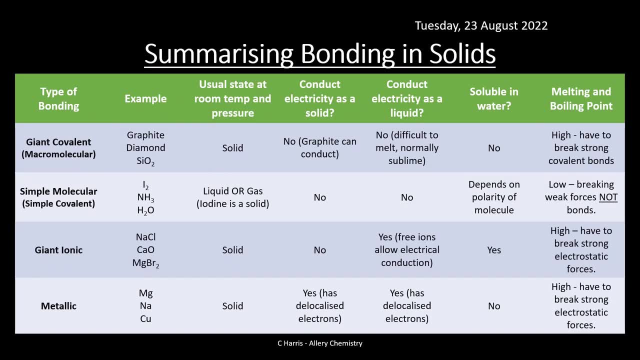 rows here really important, tightly packed together and have that form, that classic solid structure. so let's kind of summarize some of these different types of bonding again. i'm not going to go into this too much. um, there's bits in here that you would have seen from topic three, so i encourage. 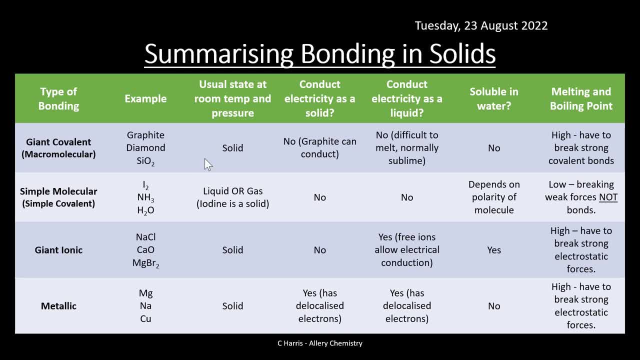 you to kind of: you know, look, watch the topic three video, really, um, but this is just really summarizing the different types of bonding in solids here that you, you really should be aware of. obviously, you've got your giant covalents, simple moleculars, giant ionics and metallics. 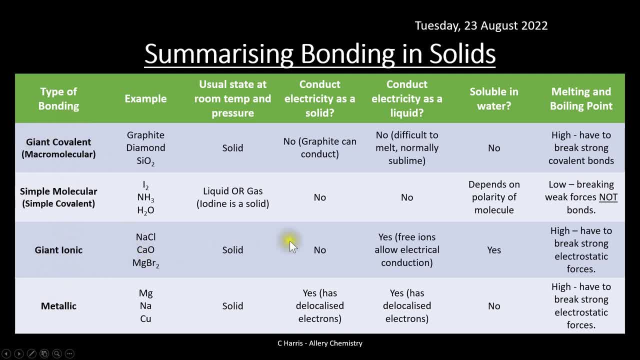 again. look at topic three for a lot more detail on these, and that's where i encourage you to look at um. you need to be aware, though, of the differences, what the difference is between these. you need to know what the state, the usual state, is at room. 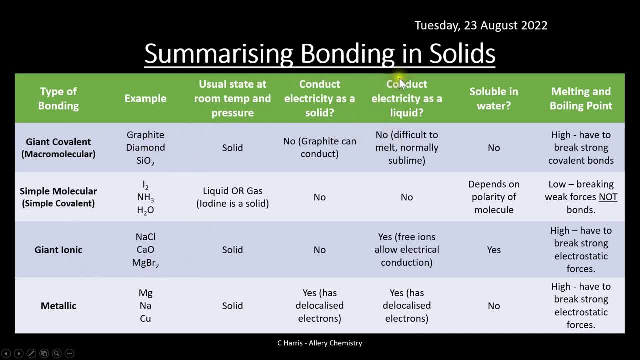 temperature and pressure. do they conduct electricity? do they conduct electricity as a liquid? for each one of these, do they dissolve in water? what's their melting and boiling points? so make sure you're aware of that as well. um just be aware as well that, in terms of solubility, um non-polar 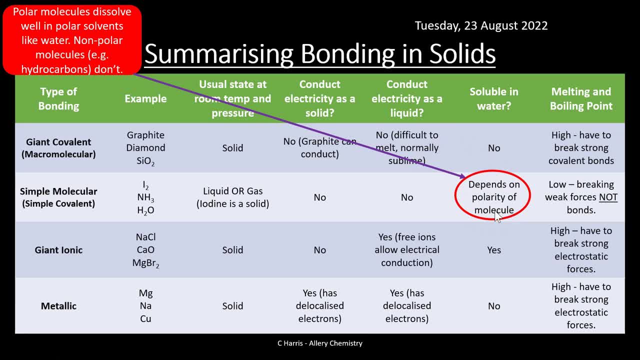 solvents or non-polar substances will dissolve in non-polar solvents. so um, for example, hydrocarbons, like cooking oil, for example, is an example of a non-polar substance, um it doesn't dissolve in polar solvents like water. so, for example, if you add cooking oil into water, it won't mix it'll. 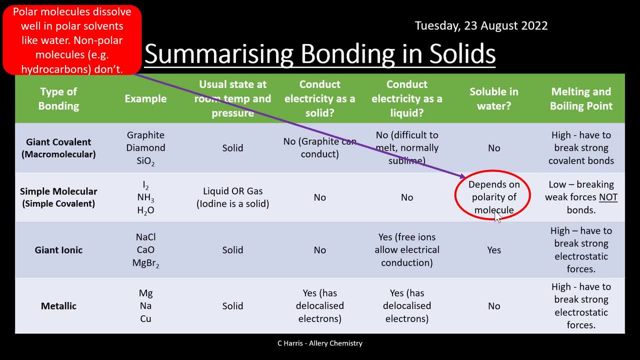 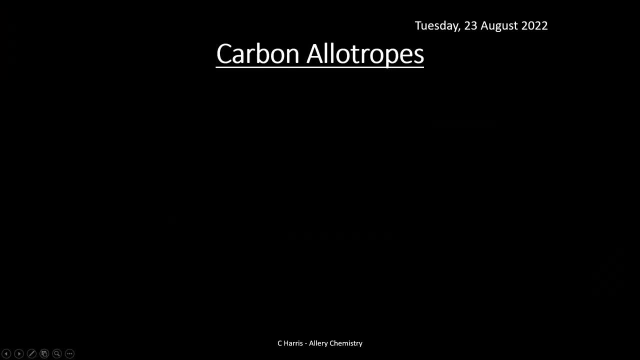 separate um but um water will dissolve um other, non other polar substances such as ammonia, for example. so so just make sure you're aware of that. but again, i'm not going to go into it in too much detail here. there is a lot more in topic three. okay, so let's look at some allotropes. um, again. 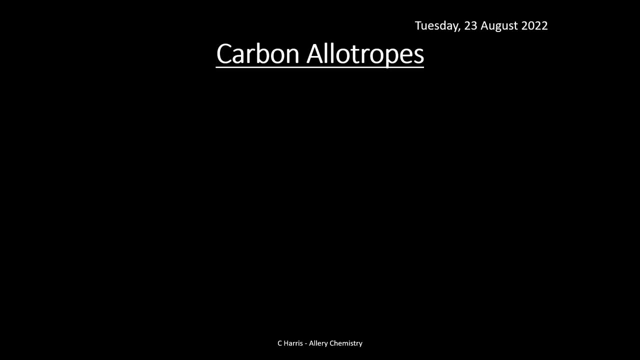 you would have seen some of these already from topic three. i suppose you haven't heard of the word allotropes, um, in in this context. so i am going to kind of bring in some of the examples from topic three into this topic here and just kind of put a different context to it. so allotropes. 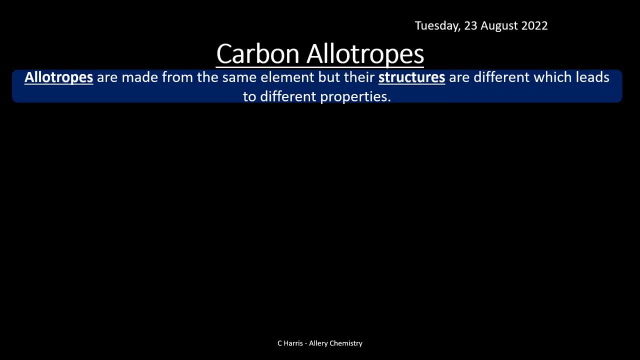 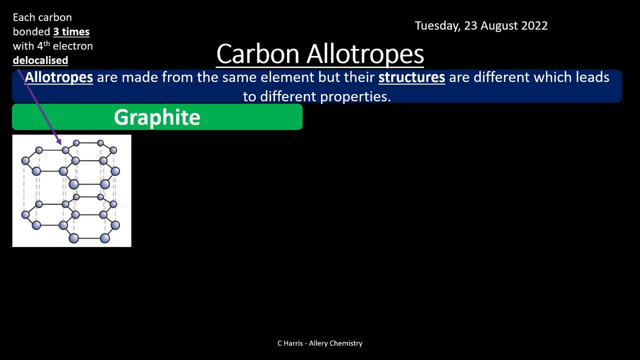 are basically made from the same element but their structures are different and that obviously leads um of of these substances as well. so one of them is um, is graphite, and again you've seen, probably seen from topic three- graphite is obviously made from carbon, um, and there's loads of strong. 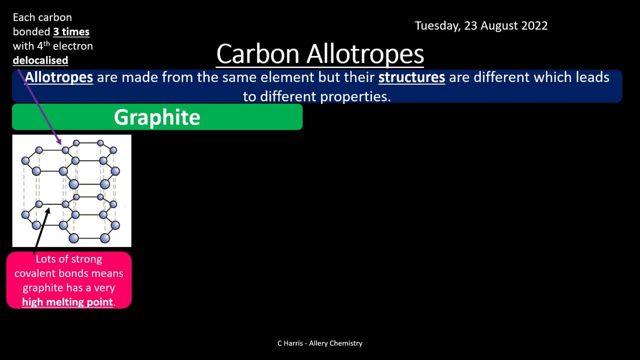 covalent bonds joining these carbon atoms together, um and in between. you have delocalized set of electrons in between layers of these carbon rings, um and the loads, because it's got loads of strong covalent bonds then um graphite actually has a really high 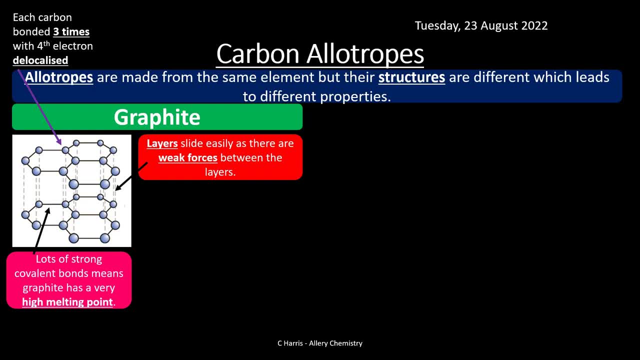 melting point now, the layers between the graphite sheets um obviously connected by the weak um forces, with the delocalized electrons, and this means the layers can slide very easily, which is just as well, because obviously, in a pencil, pencils made from um, made from graphite um, when you write, 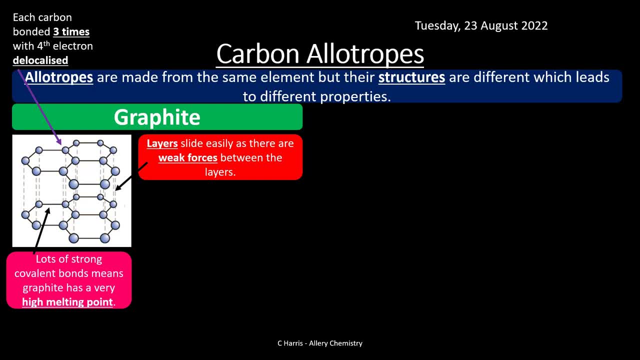 when you put a pencil against paper or you know you write against something, then basically what you're getting is is um sheets, so layers of graphite are basically coming off. um, and obviously that's quite useful, because obviously that's what you want from a pencil- um the 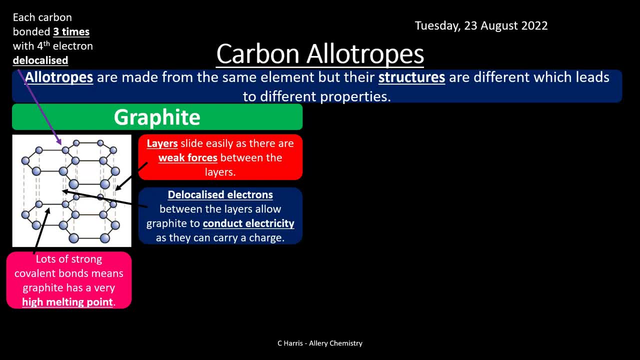 delocalized electrons in um graphite do allow um conduction of electricity, um, so obviously graphite will conduct electricity and the layers are actually quite far apart in comparison to the covalent bond length and obviously that means it's low density, so um it's quite light, which. 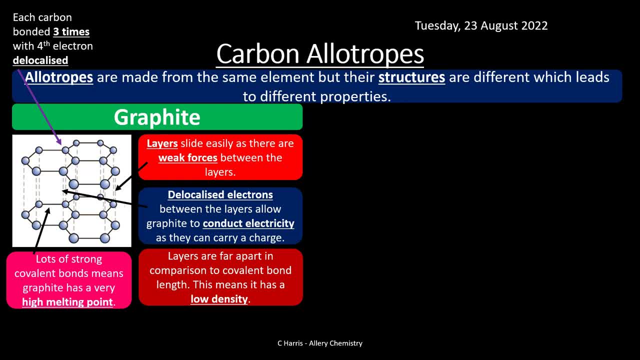 again is useful for a pencil. you don't want something that's weighs an absolute ton um, so obviously it's insoluble as well. it doesn't dissolve in water. the bonds are far too strong to break um. the other allotrope- i suppose it's allotrope, one of the allotropes, um with carbon. 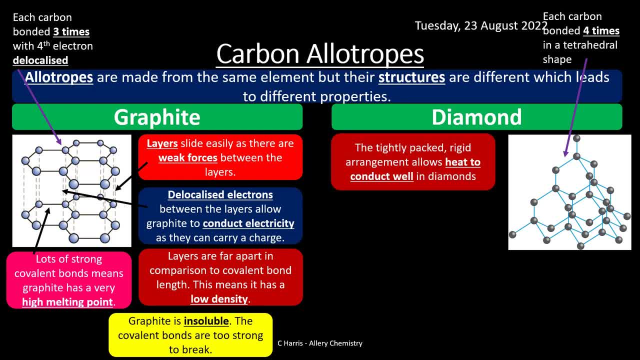 is diamond. diamond has got a very different structure to graphite. again, i'm a lot of this. you've gone through in topic three already. but it's bonded four times in this tetrahedral: um shape, tightly packed um. it conducts heat well, um, and obviously this is obviously diamond is a. 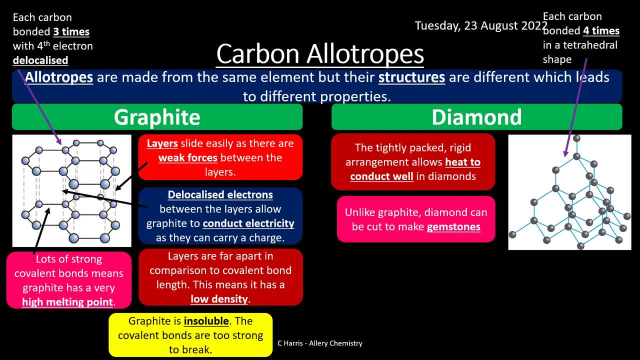 you know very good uh, so it doesn't conduct um, so it's tightly packed arrangement, it's a rigid arrangement and it allows obviously a good heat conduction um, but it's also really strong as well. it's a really tough uh material and obviously that's used in um construction, for example in. 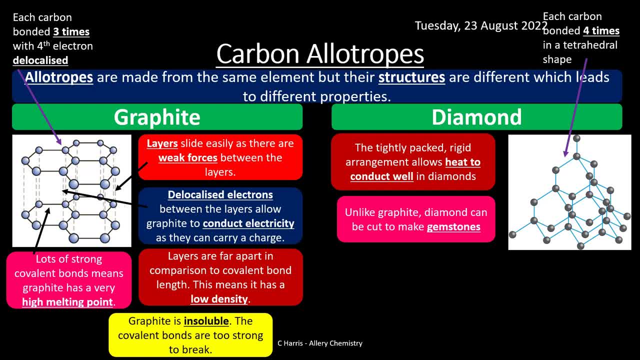 in saws, like saw blades and drill tips, etc. so you know anything where there's going to be, you know potential, a lot of heat or something which is, um, you know could, could risk, you know, being worn away. you would coat it with diamond to just toughen that up a little bit. um, the unlike. 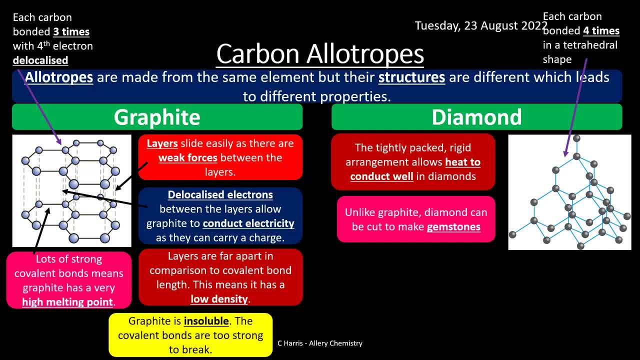 graphite. obviously diamond can be cut to make gemstones, so it's it's holds its shape better than graphite. to that extent, when it's cut, obviously an incredibly high melting point. it's got so many strong covalent bonds on there so it's a very hard substance and it doesn't 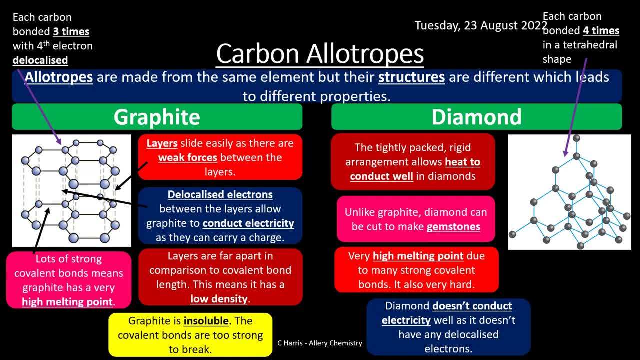 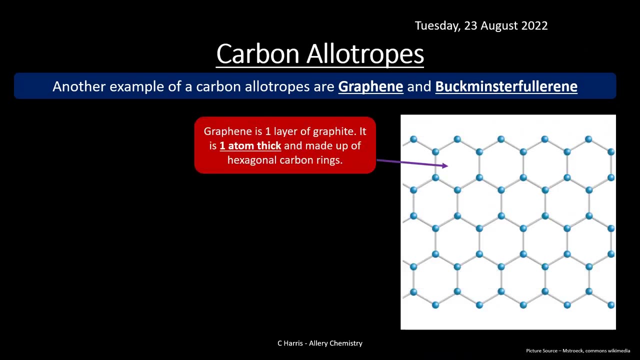 conduct electricity, um, you know at all, really, it doesn't have any delocalized electrons at all, um, unlike graphite which does, and obviously, as you probably expect, it is insoluble in water as well, because the bonds are too strong for water to break apart. okay, some other ones, some other allotropes, um, which you may not have heard of before me. i may. 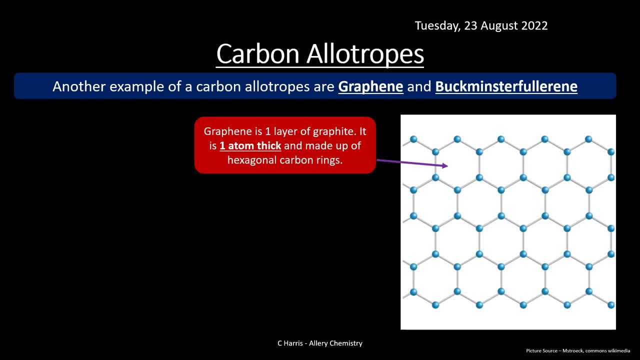 not have done. um graphene is is quite a um a revolutionary material actually, and i think it's obviously it has changed the way in which particularly mobile phones, for example, and technology, so modern kind of um digital technology, um graphene is used quite. you know relatively quite a lot, but i think we can expect graphene to be used extensively in future technology as well. 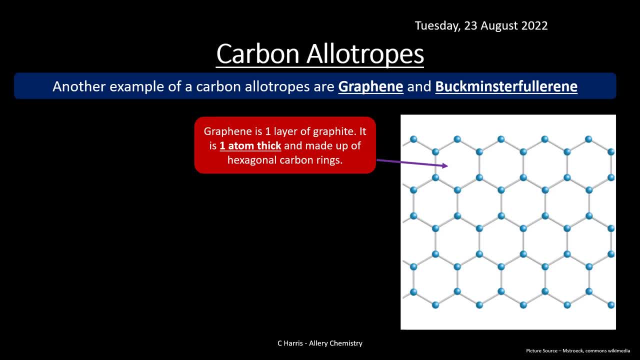 um, you know, when continuing in with that, graphene is just basically graphite, but it's just taken one layer of graphite um, it's one atom thick, so it's incredibly thin. um made of hexagonal rings, that's. that's basically all it is. um, graphene is really lightweight and it's transparent and it makes it great for um anything that has to. 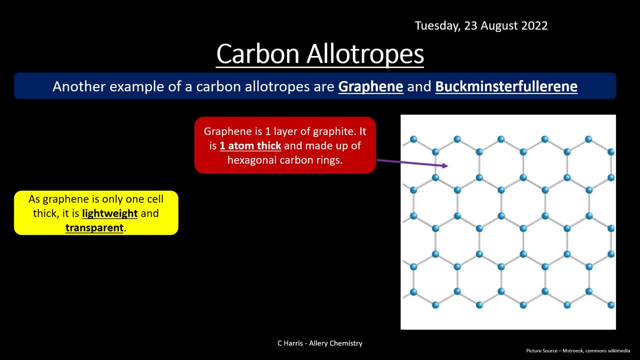 be carried around. anything that doesn't shouldn't really be too heavy anyway. if it's light, it's a good thing. it's transparent, so that could be used, for example, on monitors and screens and things like that. so touch screens, for example. um delocalized free moving electrons makes it a 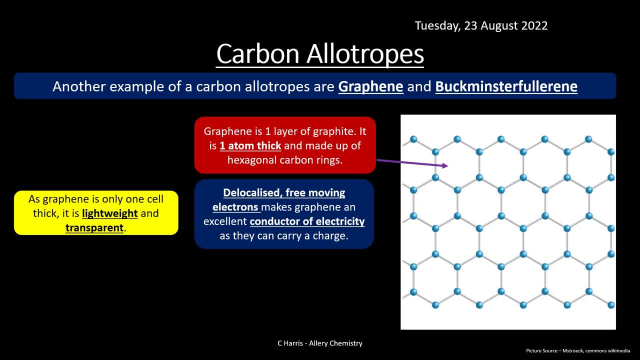 really good conductor of electricity. so that's good because it's used in electronics, as i mentioned right. as you can see, um, and it's got this delocalized electron kind of sea of electrons as well. um, that's strengthened um, so the same, obviously, delocalized electrons strengthen the. 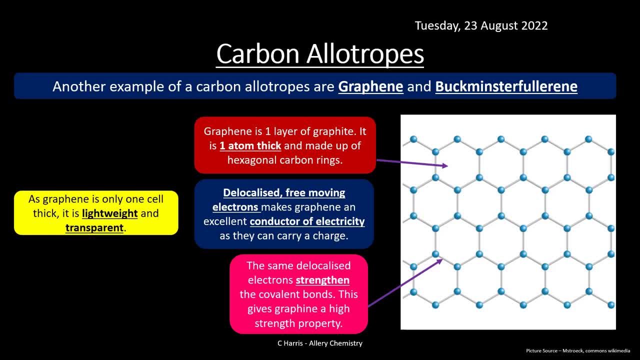 covalent bonds and this gives graphene a really high strength property, so it can be really robust and it can be used, for example, to strengthen materials. it might be in cars, it might be in- um, you know, materials around the house. it's lightweight and strong, is a really good property. 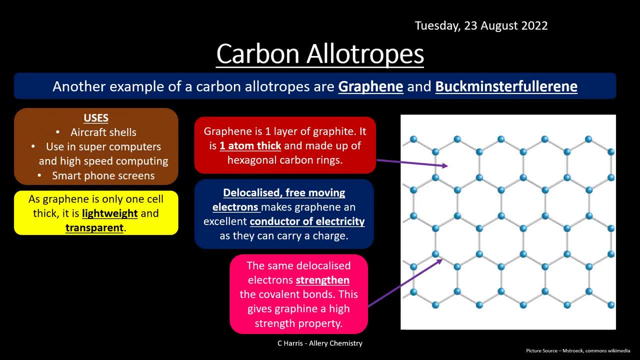 to have. you can see, you know it can. you can come up with quite a few uses here. so, like i say, some of the uses are smartphone screens- i mentioned before- and supercomputers. so they can. they can transfer a lot, of, a lot of electricity, a lot of data very quickly and aircraft shells. so if you 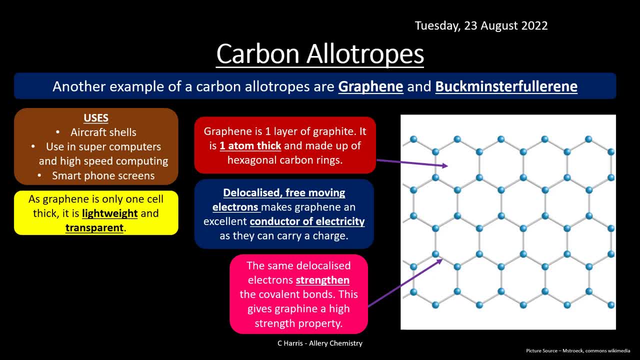 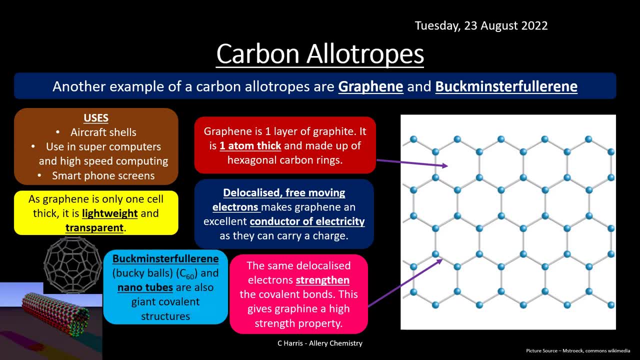 make planes lighter. they use less fuel and you could probably go further, because they don't have to carry as much fuel, or the body, main body of the airplane is as light as it can be. um buckminster fullerene is another one other also known as buckyballs, um. so buckyballs are um carbon uh. 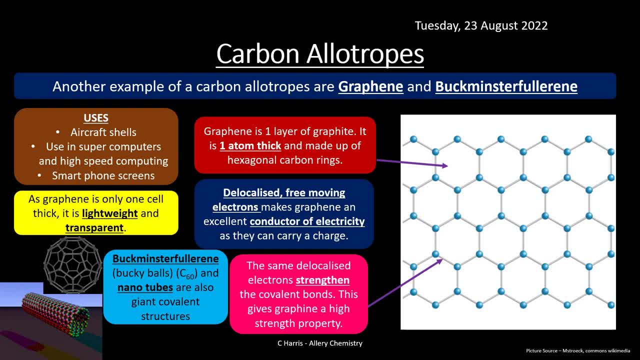 carbon atoms and you've got 60 carbon atoms arranged in a football type structure. um, again, um, they're giant covalent structures. they're used in a medicine. um, this is probably gonna be one of the next biggest areas of medicine and the drug, drug delivery and development and whereby you can 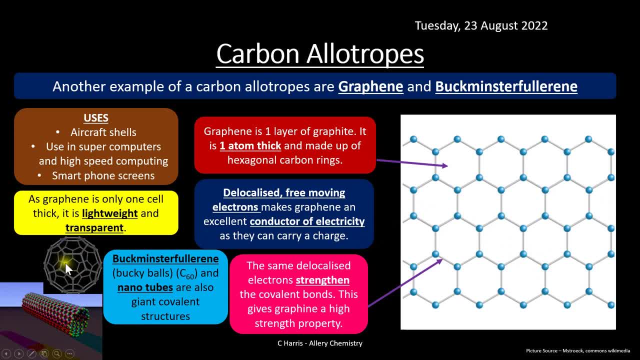 put a medicine in a, in a like a cage, like this, like a buckyball, and that cage can then open up when it's delivered to a particular site. so, for example, cancer treatment. this could be quite revolutionary in that, in targeting specific areas, for example, cells, cancer cells rather than, um you know, at the minute, although we do have, 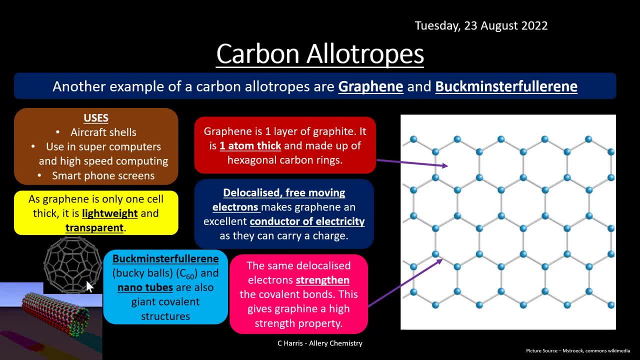 specific drugs that target specific cells. they are starting to come through um. generally, the treatment is quite generic and it can affect other cells um as well and can make people quite ill. actually, the treatment is quite generic and it can affect other cells um as well and can make people quite ill. actually, the 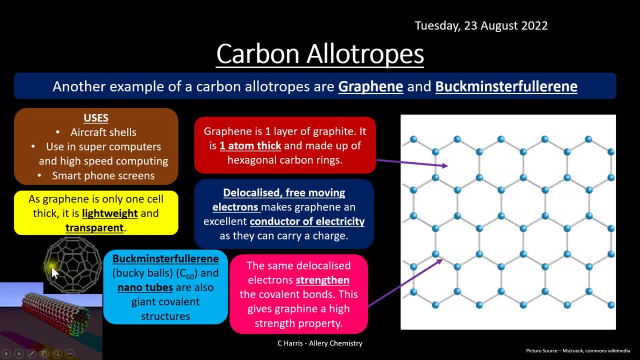 treatment itself can make them quite ill because it's not specific to that area. so this is a huge area of science where, um, you know, chemistry like this- so buckyballs and you know, and c60 and nanotubes and things like this- can help, really help revolutionize in particular areas of medicine. 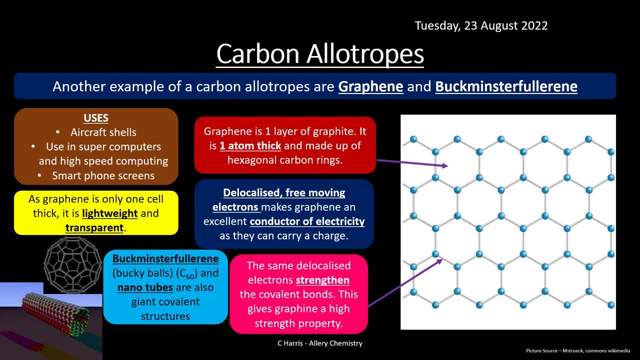 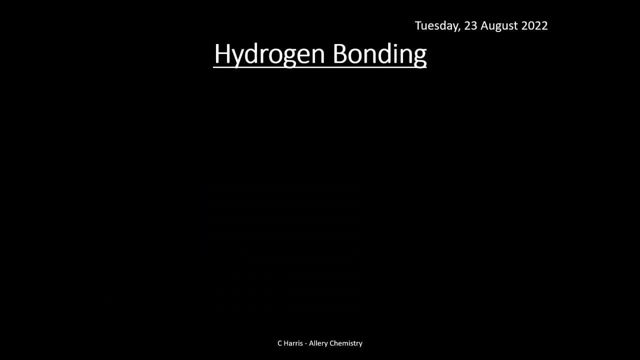 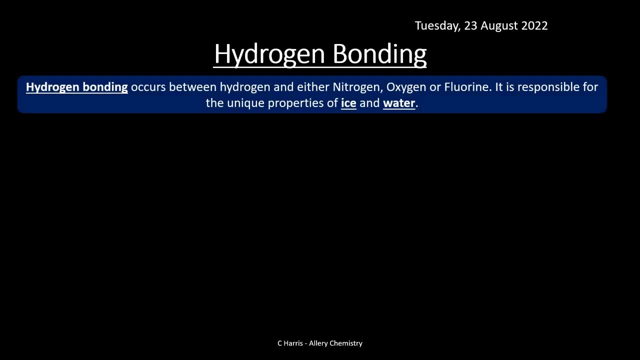 but obviously you know um areas of technology as well. so big, big areas, something, something like carbon and the way it's structured, can have big, uh, big differences, um. so the other type as well is um, hydrogen bonding, um. so obviously we need to be aware of that. now you again you had 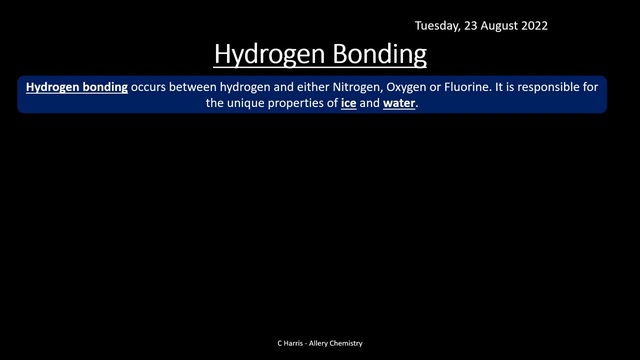 seen some of this in in topic three. i suppose this one just goes into some more specific examples here. so obviously, if you can remember from that topic, hydrogen bonding occurs between hydrogen and um, three of the most, some of the most electronegative elements in the periodic table. 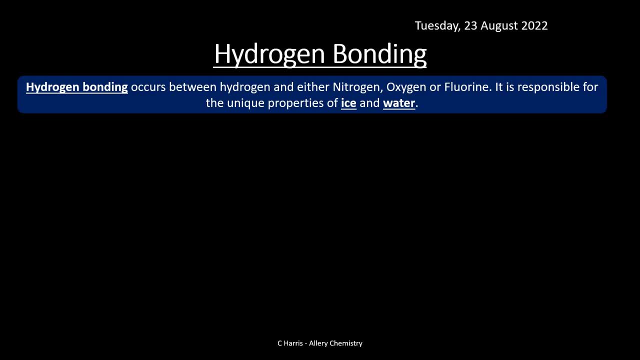 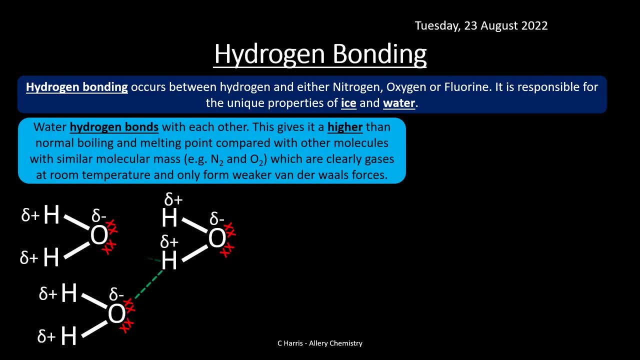 and that's nitrogen oxygen, fluorine, um, and it's responsible for the unique properties of ice and water. okay, it's quite an interesting topic, this. actually there's loads of different kind of things which you can kind of see in everyday life, but um. so basically you've got water molecules here. 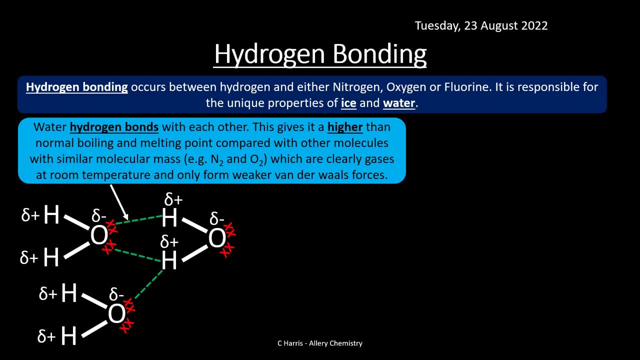 obviously we knew from the previous topic that they form hydrogen bonds with each other and that gives them a higher than normal boiling and melting point compared with other molecules with a similar molecular mass, such as nitrogen and oxygen. so water is not exactly a big molecule at all, so really it shouldn't have very strong forces, you know, compared to 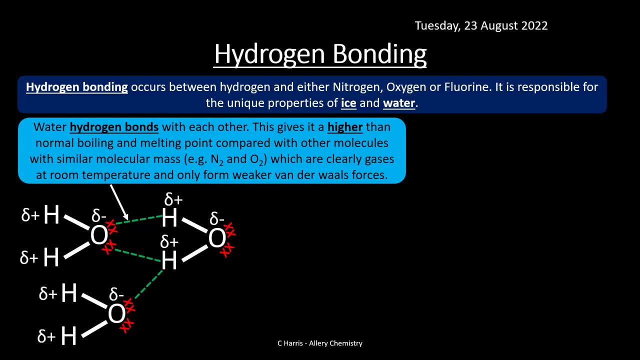 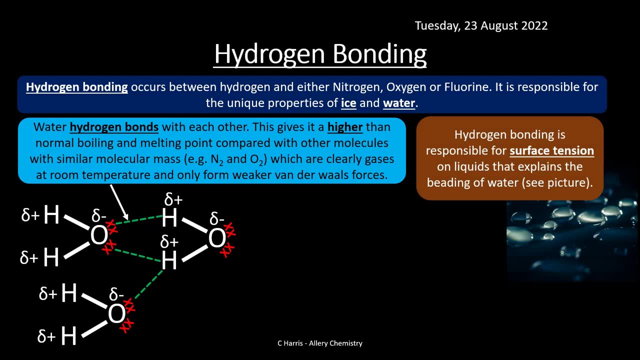 its, you know, molecules of a similar size. but they do have this, obviously, this property that they can hydrogen bond, which gives them a bit of a different, um, you know, a different, uh uh, different properties to their, you know, to molecules of a similar size. so hydrogen bonding is actually. 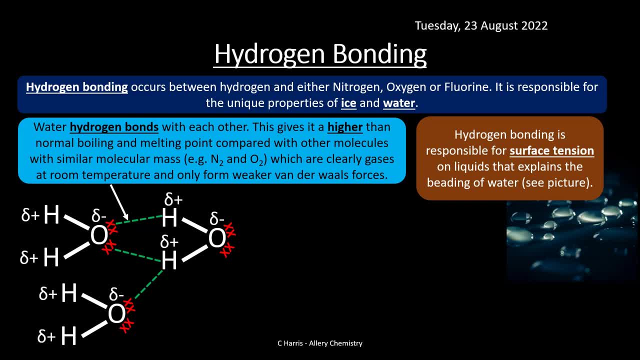 responsible for um, surface tension, um on liquids, and that explains why we get water that beads. now, if you look at, say, if you've got a car that's just been lovely and waxed, been lovely, valeted, it's got a waxed water, it's got a waxed water. it's got a waxed water. it's got a waxed. 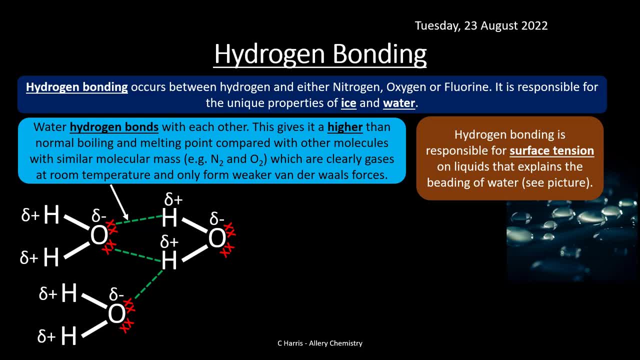 on it and then, if you tip water on that wax, the water will bead together. it'll actually clump together. instead of being spread out, it actually beads together and collects in one place and water has a tension- that is a surface tension, and this hydrogen bonding is responsible for creating that. 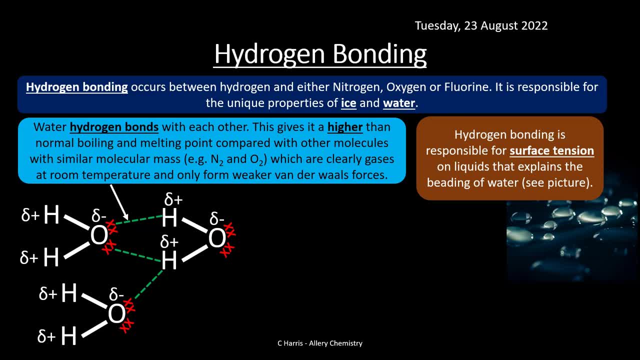 that? um that surface tension, you get certain? um insects that can skate across the top of the water. they can sit on the water because there's a surface tension there. also, if you look at divers, there's been the? um the commonwealth games, um, that's been on recently. so you know, if you look. 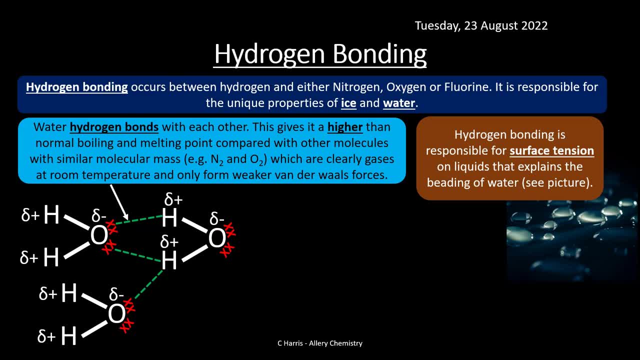 at divers when they try and dive in, they'll dive obviously with their hands outwards so they can kind of glide into the water. if you try and dive and do what like a belly flop as opposed, and go in a bit like a starfish, that's going to hurt quite a lot because the tension on the surface of the 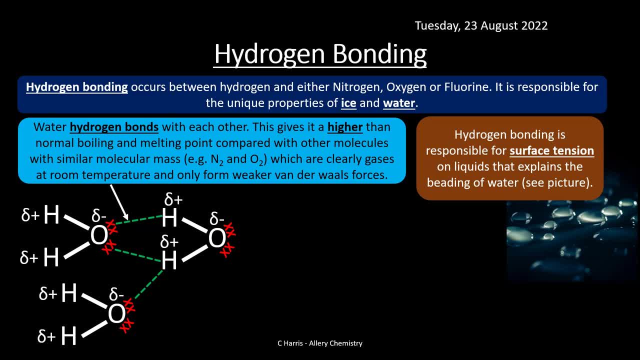 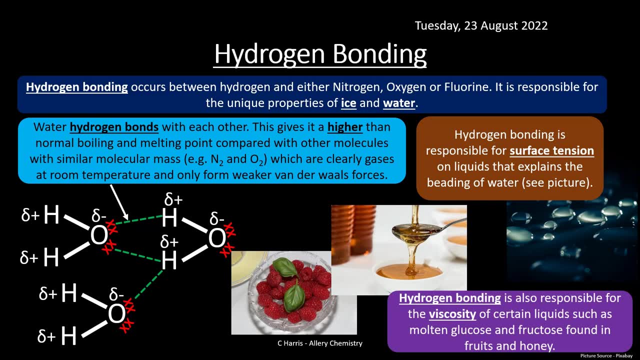 water applies a force against the body which will hurt and um not really advised because you could get winded. actually, if you do that, so don't worry about it if you don't want to do that. um. so hydrogen bonding is also responsible, obviously, for viscosity of certain liquids, so 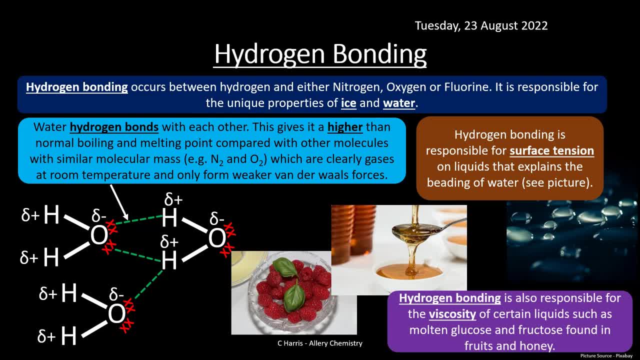 for example, um molten glucose and fructose, and that's obviously found in fruits and honey. um, so obviously the reason why they're quite um viscous, which just means thick um, is because of the hydrogen bonding between the molecules. so it just holds its form quite well. treacle is a good. 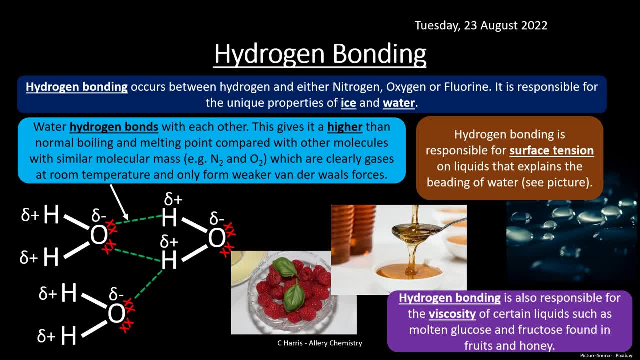 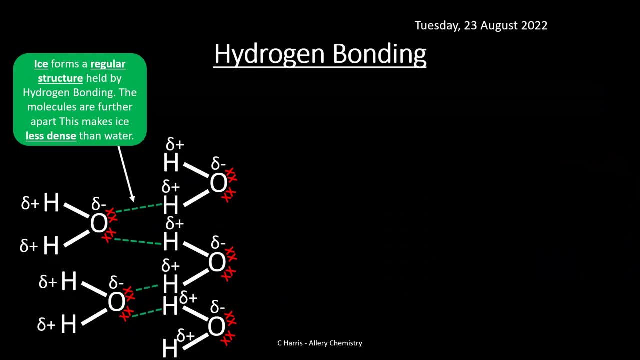 example of that. it's just sugar that's been obviously refined and and um put into a liquid liquid form. so just looking at a little bit more, i suppose a little bit more detail into hydrogen bonding if we just come back onto water and in particular, if we look at ice- now, ice is one of these bizarre. 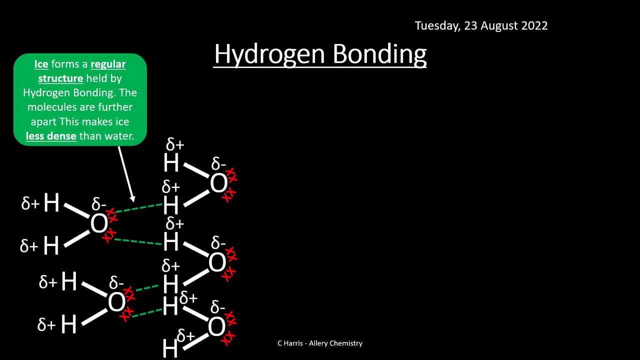 um, well, a bit of a bizarre um entity, i suppose, because if you look at um uh, other solids or liquids, when you cool them they normally contract, they take up less space, and when you heat, um say, a solid or a liquid, they expand. so when you heat a solid in particular, they expand and take up more space. 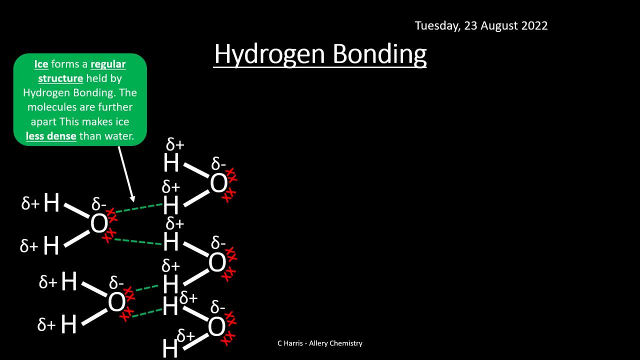 now, water is a bit weird because when you cool it down, it actually gets bigger. ice takes up a larger amount of space than its liquid form, and which is which is weird, and this is down to purely down to hydrogen bonding, um, and to an extent where water is actually less dense than as a solid, than what? 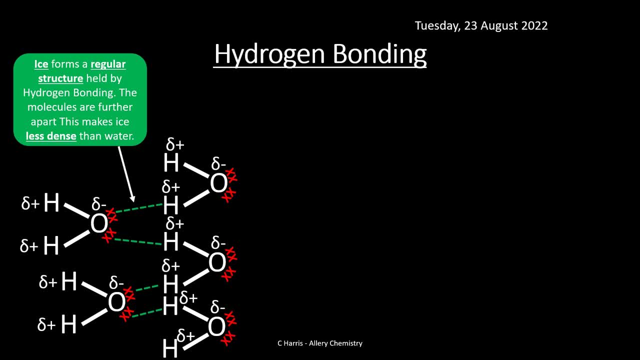 it is in liquid form and that is why ice cubes float on top of water, because they're denser and the density decreases as you cool them down, and it's thanks to hydrogen bonding that kind of separates the molecules out and arranges them into a regular arrangement. um, but they're kind of more. 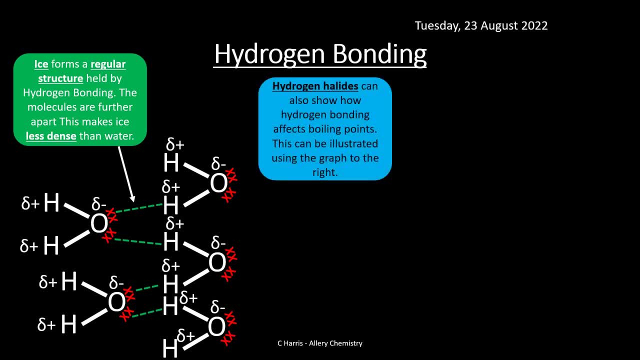 separated out than what they were as a liquid, um, and obviously that obviously transpires. you can see ice floating on the water and hydrogen halides, um, so can also show how hydrogen bonding affects boiling points, and we can use a graph to eventually look at the difference of these as well. so this 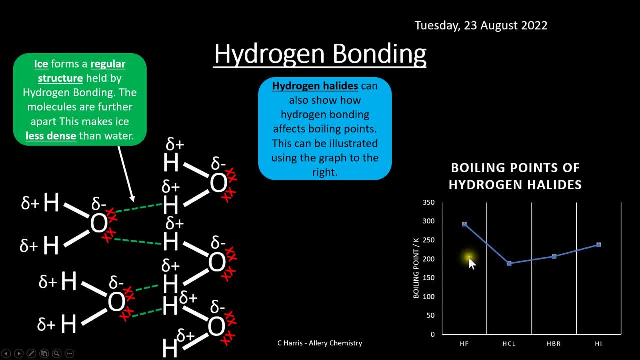 graph here has got boiling points and we can use a graph to eventually look at the difference of boiling points in kelvin- um. let me bring the mouse in there. we are so boiling point in kelvin- um and you've got um hydrogen fluoride, hydrogen chloride, um hydrogen bromide and hydrogen iodide. 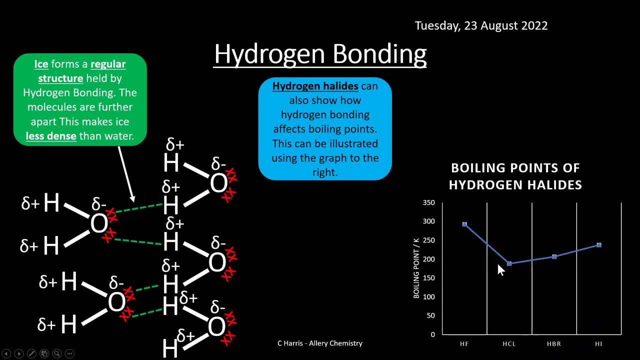 so this is basically going down group seven, which you'll see later on in year one. so there's bits here. we can see there's a lot of crossover, but basically it's looking at the boiling points of each of these different substances here and what they are you know over time. now one of the biggest, 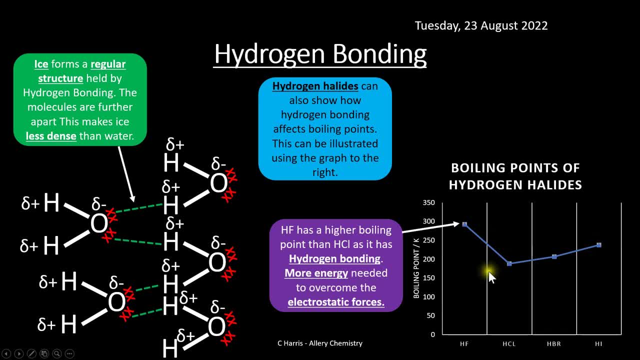 things to note is obviously here. treff has got a higher boiling point in any of these substances than any of the other ones, despite the fact that it's quite small. but hf can hydrogen bond um, and so more energy is required to pull hf molecules apart than it is for hcl, hbr, hi, which 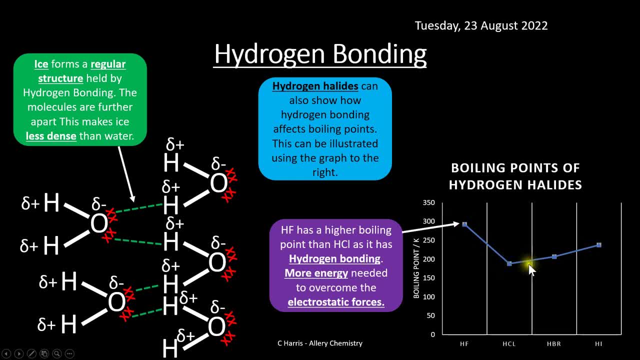 only have permanent dipole dipole interactions. they don't have hydrogen bonding and, if you remember from topic three, permanent dipole dipole forces are weaker than hydrogen bonding, and so that's why these boiling points are lower than what they are compared to compared to hydrogen bonding. 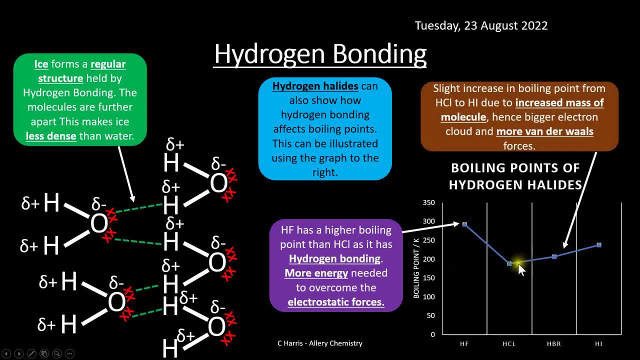 hf. there we are. okay. um, some of these may have as we actually go along here as well. so hi doesn't really have that much of a difference in electronegativity. so all of these will have van der waals forces as well. but, um, this hcl will have the permanent dipole dipole, less so with some. 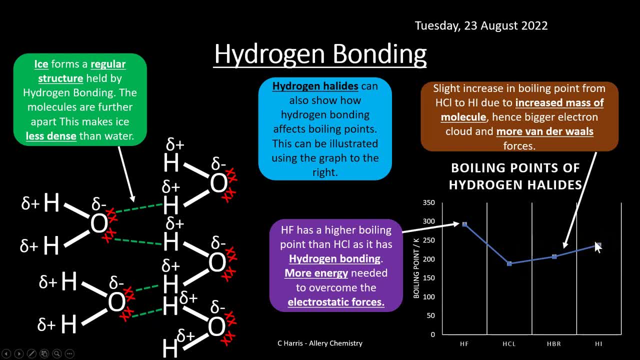 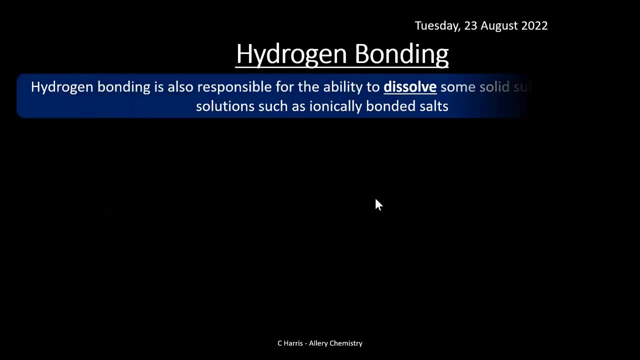 of these, for example, hi, there isn't much of an electronegativity electronegative difference anywhere between hydrogen and iodine, so yeah, so hydrogen bonding, obviously um does have an impact in terms of the melting and boiling points of these substances. okay, so let's look in at um some um other examples of hydrogen bonding. um, this is obviously also. 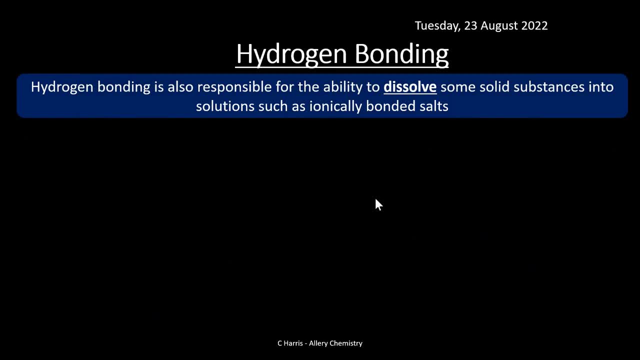 responsible for the ability to dissolve some solid substances into solutions. um. so ionic salts, for example, are a classic example where salts are pretty soluble- um, a good chunk of them anyway are, and they'll dissolve in water. and the reason why salts can dissolve in water is actually because water can hydrogen bond, so you can see how important water is. 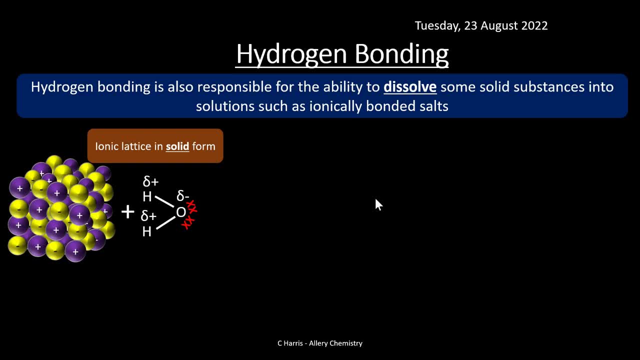 actually, in chemistry, you pretty much dissolve everything in water, to be fair. so let's have a look at this then. so we've got your ionic lattice, so this is your ionic compound here. so you might have seen this again from topic three, um, you've got your um positive and negative ions that have 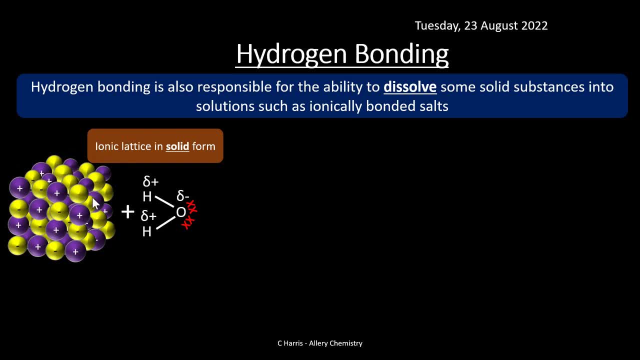 obviously formed in a giant ionic um substance, giant ionic compound, and you've got your water molecule here with your polarities on there. so if what happens is actually the substance, the bonds are broken to create free moving ions, so these ions are then broken apart. so this is when you um, when you basically add it to the water. 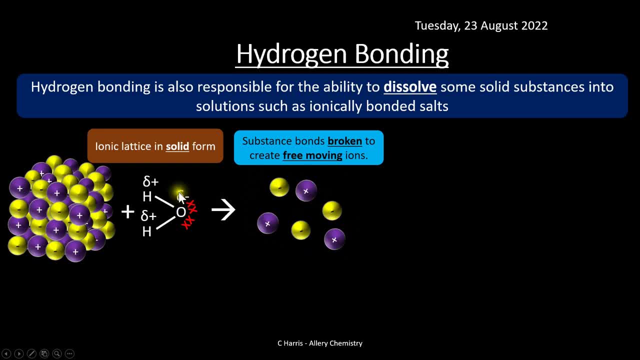 the ions start to break apart, um like that, because obviously the charges on the, the uh, hydrogen and the oxygen, um, and obviously the hydrogen bonds, it then dives straight in um and the um, the um, the water starts surrounding the individual ions and we say these are hydrated and this is effectively. 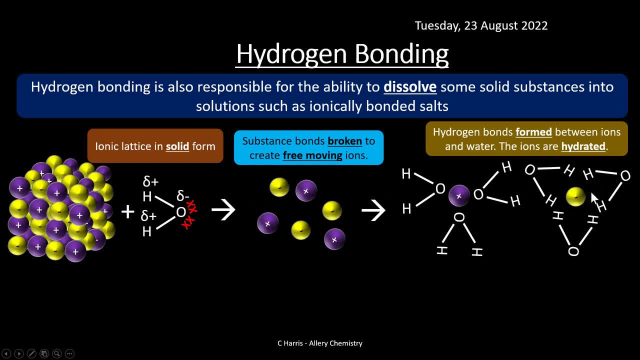 we're dissolving the salt into uh, into um, into water, effectively so and it's the hydrogen bonds that exist between obviously, the. the delta negative oxygens here are attracted to the delta, to the positive ion- sorry, um- and the delta positive hydrogens are attracted to the negative. 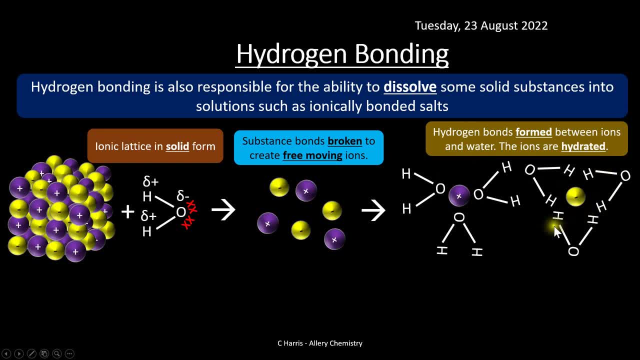 ions. now they keep these ions apart and that's effectively what allows water to dissolve in the water. to uh, what allows salts, should i say so ionic compounds, to dissolve into into water? so, like i say, most ionic compounds do do this and obviously we've seen the structure obviously starts to break. 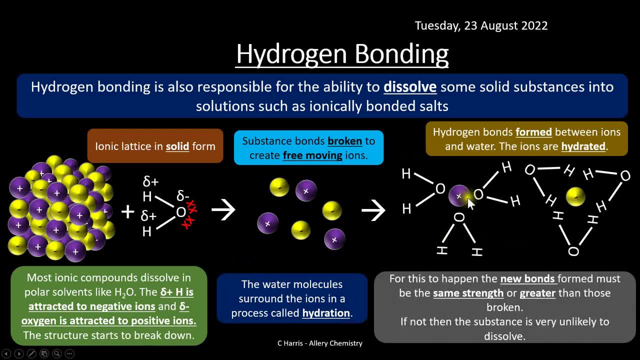 down, um, and obviously they surround the ions and we call that hydration. and obviously for this to happen- not because not all salts are soluble, um, but so for this to happen, the new bonds formed here, so these interactions here, must be the same strength or greater than the ones that we use to. 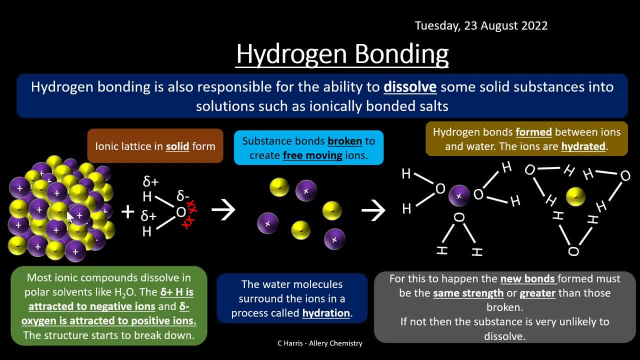 down in the first place. if not, it's not likely to dissolve. and actually sometimes, um, you'll know in, you know, if you do any form of cookery or anything like that, that sometimes you want something to dissolve, you might have to heat it up, you might have to give it some energy to to kind of help it. 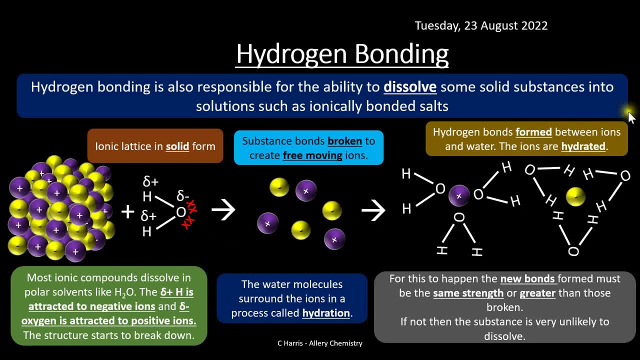 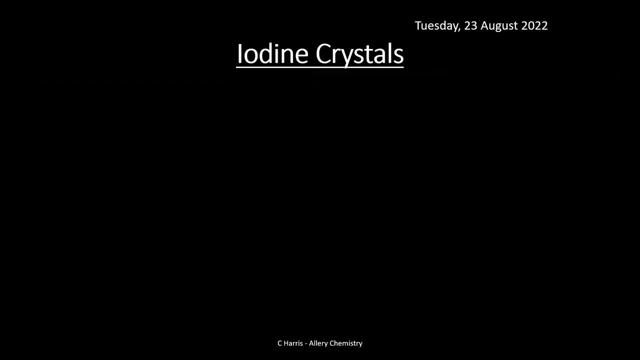 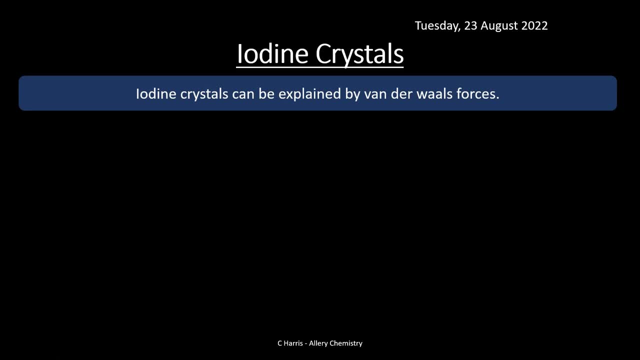 break apart, okay, so, um, let's look at the um, i suppose, another example, which is iodine crystals. um, just looking at another example of solids. so obviously these can be um iodine is a bit of a strange one because um iodine is, um is a solid. 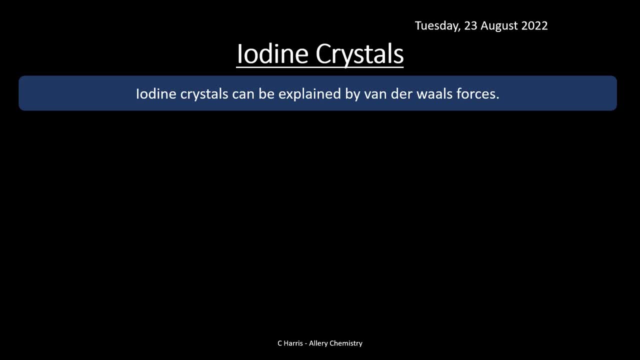 at at room temperature, but actually when you heat it up at room, uh, room pressure, um, it actually sublimes. it goes straight to a gas. it doesn't actually go to a liquid, um. but what we need to do is basically understand the structure of of iodine and again, from topic three you'll understand. 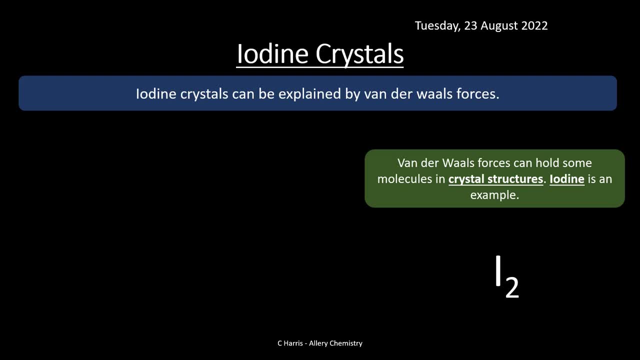 that van der waals forces are the weakest type of forces in America. so we're going to look at molecule and iodine just has van der waals forces. there are no other forces there, um, but these forces actually help iodine to form a crystal structure at room temperature. um, so iodine uh. 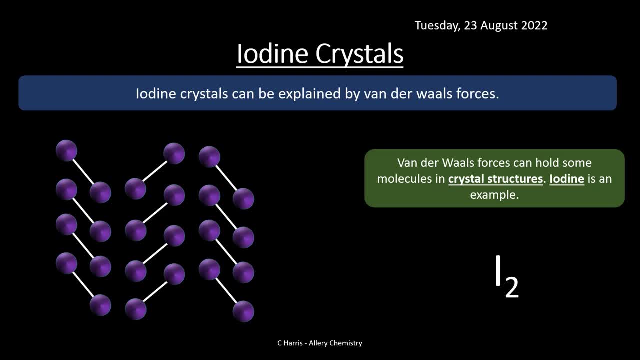 there we are. so iodine is a is a nice kind of um. it's a gray, grayish, purplish um, solid at room temperature, uh, and it's crystalline. it looks like crystals, um, and crystals means that you have um, you have a regular arrangement of molecules. obviously it's a solid, but it's not a solid. 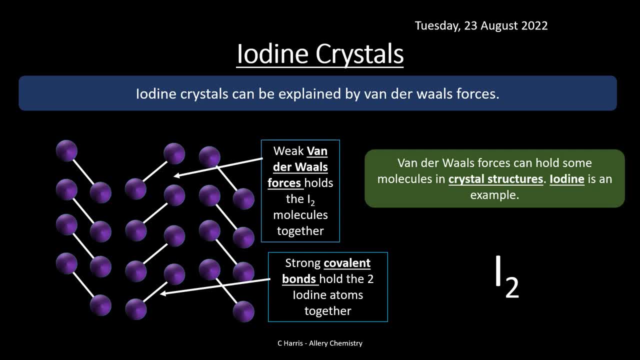 but you have these weak van der waals forces um which hold these iodine molecules together in between the atoms, though just to make a distinguish the difference between them, you have strong covalent bonds that hold the two iodine atoms together as well. so it's the um weak. 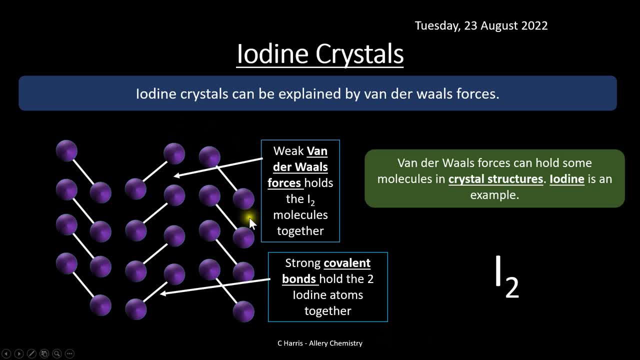 forces though that hold iodine as a solid together. so just make sure you're aware of this and you can kind of describe the difference between the forces and the solid and the weak forces between the molecules, um, which are these here, and the bonds that exist between atoms and and the 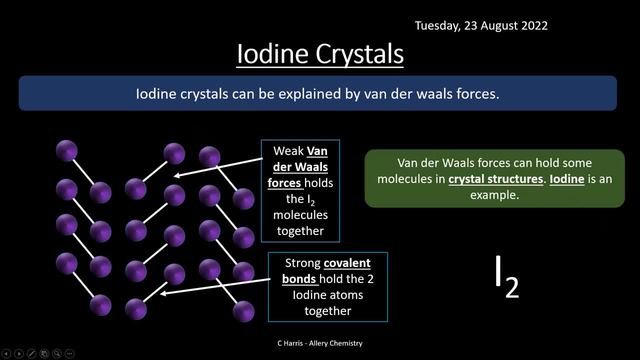 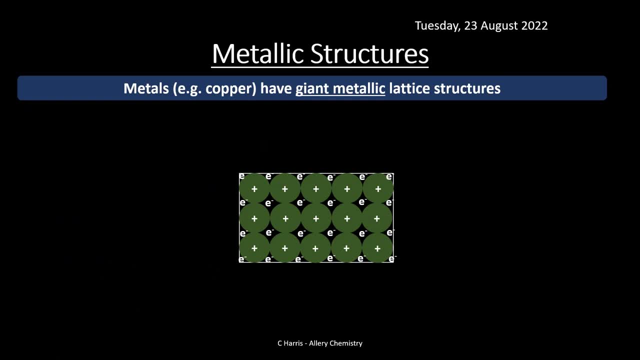 reason why, obviously, iodine is a, is a solid, okay. and then just the final bit really is metallic structure and again you would have seen this in topic three and i urge you to kind of look at topic three or watch the topic three video for a little bit more detail on this. but just briefly. 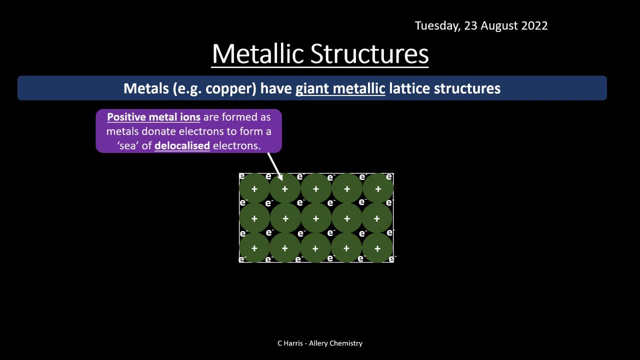 just to run through the metallic structures. obviously metals um are solids, they will, most of them are, apart from mercury um. but you know, for the purpose of this they're solids, they have that positive metal charge with a delocalized sea of electrons um they, um they are obviously have this electrostatic attraction between the positive 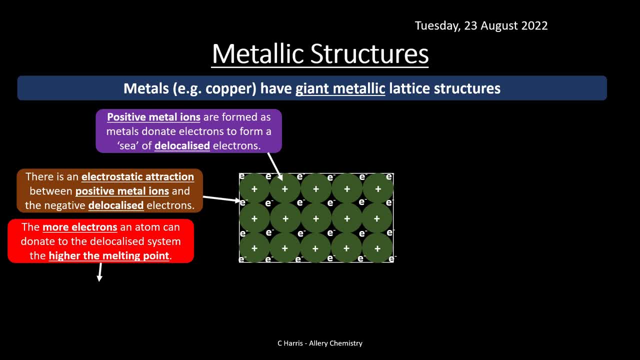 charge and the negative electrons, um the more electrons you have between the metal ions, um between the metal ions and the electrons. obviously, the more electrons that are floating around, the stronger that electrons are and the more electrons that are floating around, that attraction is and that can be classically seen. with um sodium can give up one electron. 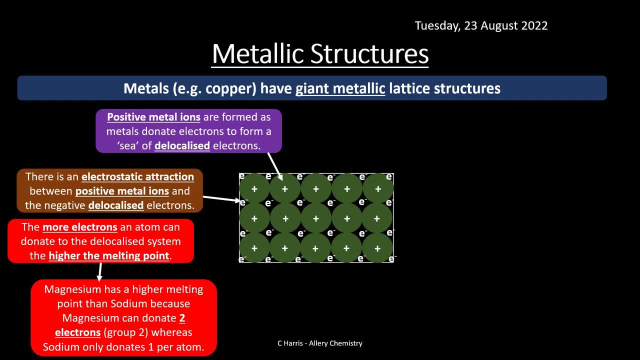 in the metallic structure, whereas magnesium can donate two electrons per atom of magnesium um. magnesium is a higher um boiling point, or higher melting point, should i say, than sodium. sodium is quite soft. you can actually cut it with a knife. it's like butter. it's a bit bit weird.